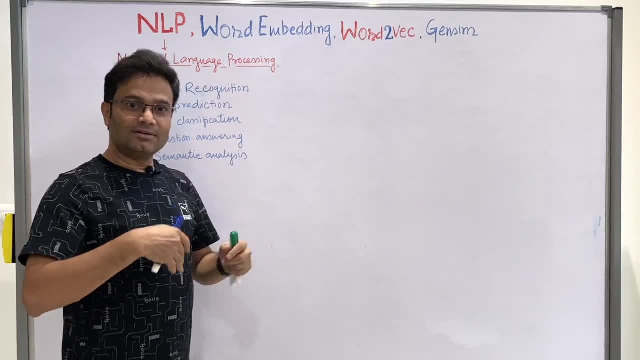 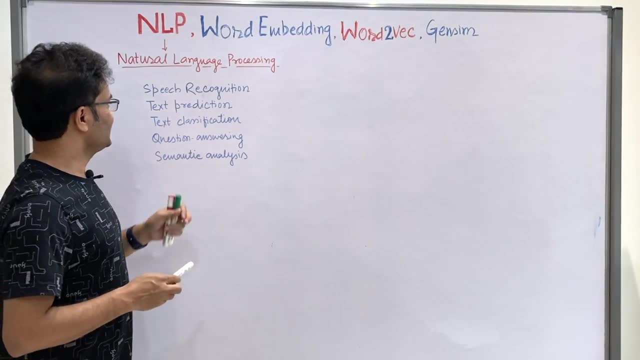 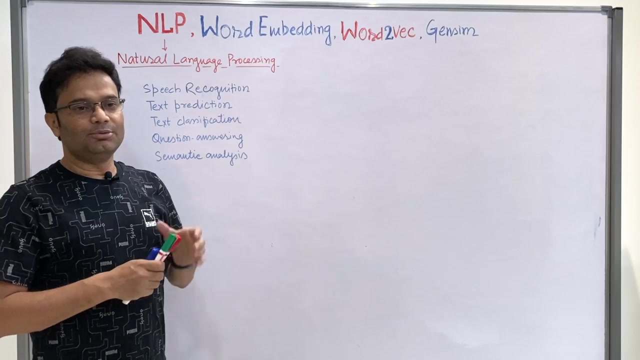 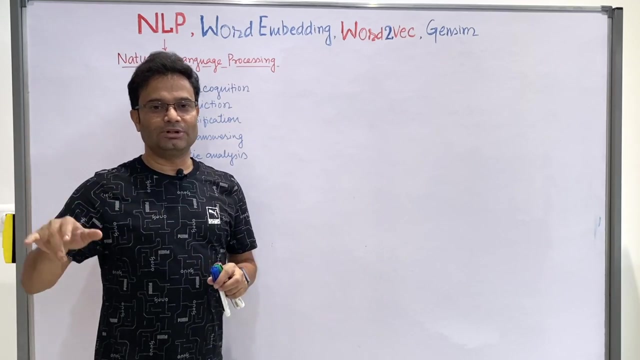 is going to understand your voice. So NLP is there. This text prediction: Nowadays, you have already observed when writing the email, particularly in the Gmail, if you write some sentence after that they start predicting some words. So you no need to write, you can just put the enter and the predicted sentence. 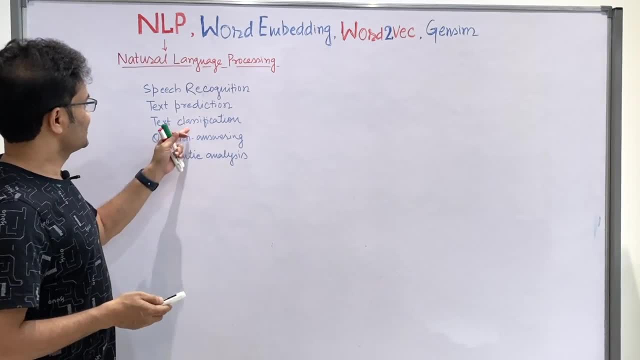 words make your sentence complete right And the text classification. So if you go in a new China and they develop a new JavaScript, if you go in a new channel, you can create new Informations, right? And then there are some, Yes, there are some, So you can run. 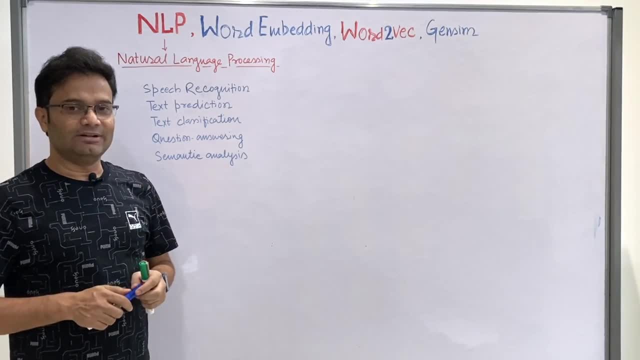 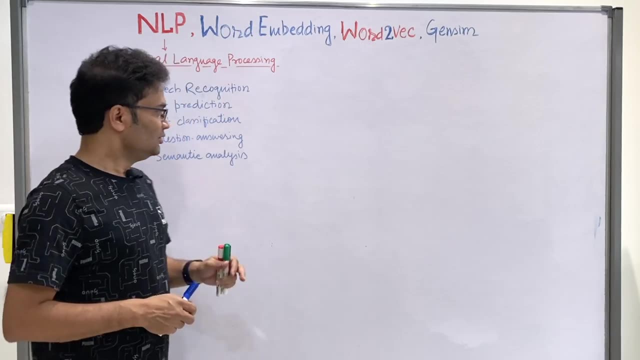 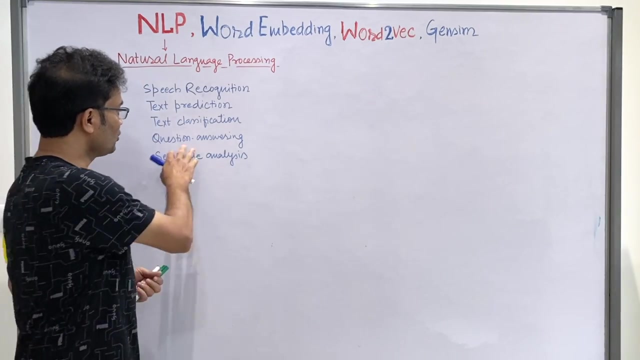 divide or categorize the news in the different category: right. So you have some politics news, sports news, world news, finance news, how they used to do that. So behind that we have the test classification that also we can achieve through the NLP. 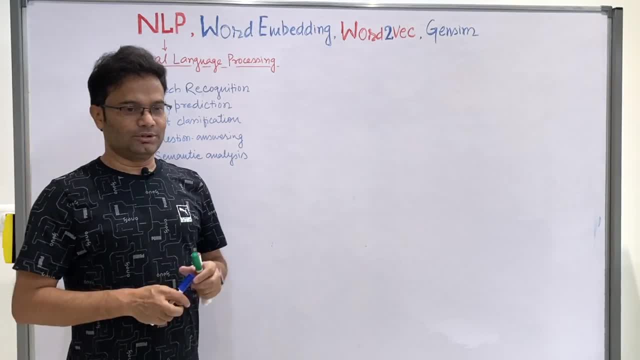 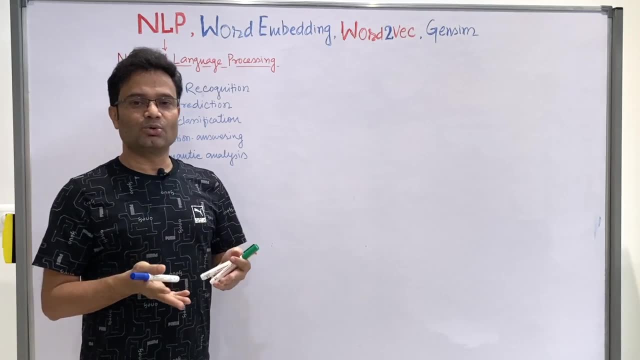 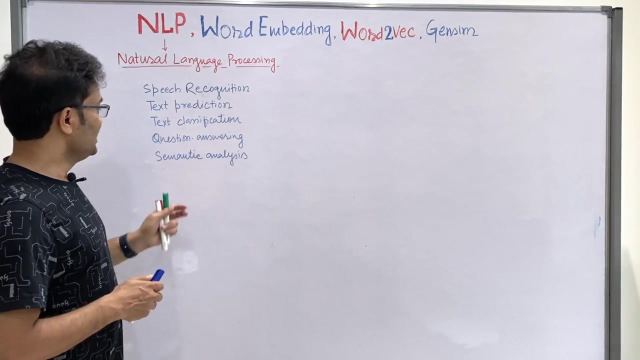 Questioning answers, right. many website implement the chatbot. if you give some questions, they will give the answer. So how those chatbot understanding your questions? even you write your questions in the different, many other ways, right? So that is also the one of the NLP use case. 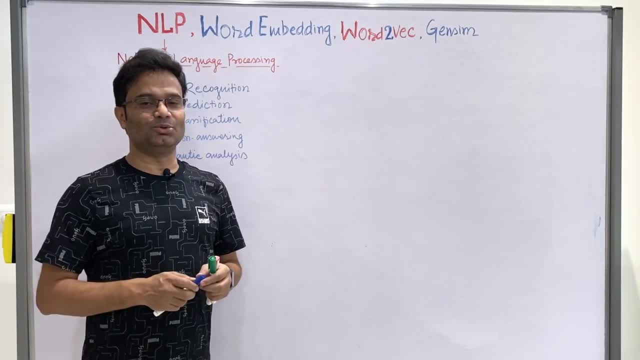 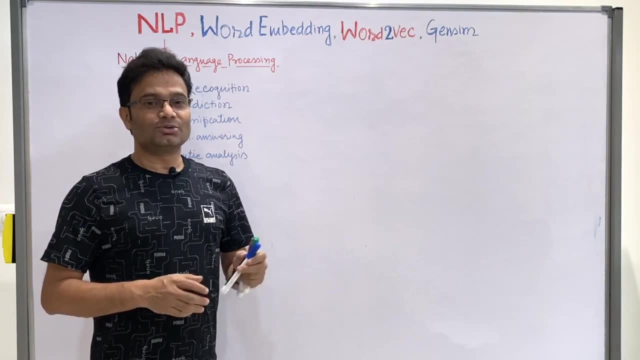 Semantic analysis. right so now it is very famous to know the review. even if you go to purchase some product on the Amazon or any website, you want to see the review, right. So how we analyze the review, whether this is negative review or the positive review. 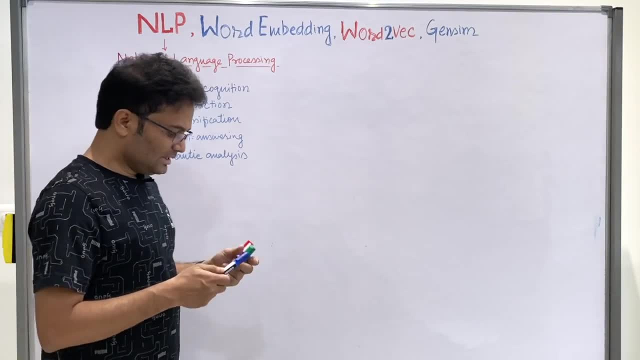 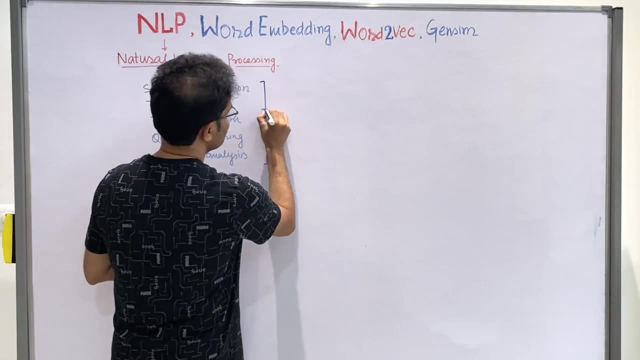 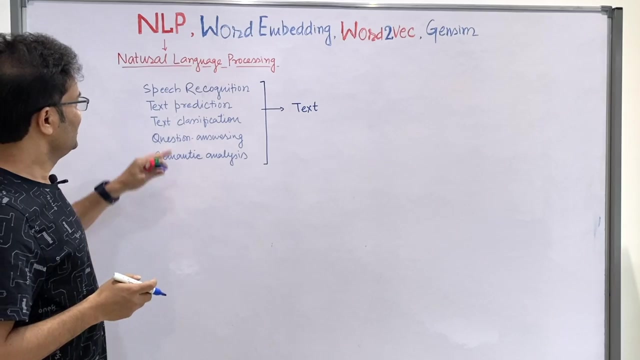 all those things come under the NLP. But if you see that, For all the use case, what is the input in the system? the input in system is the text, Even for the speech recognition. your speech convert into the text, right and everything. 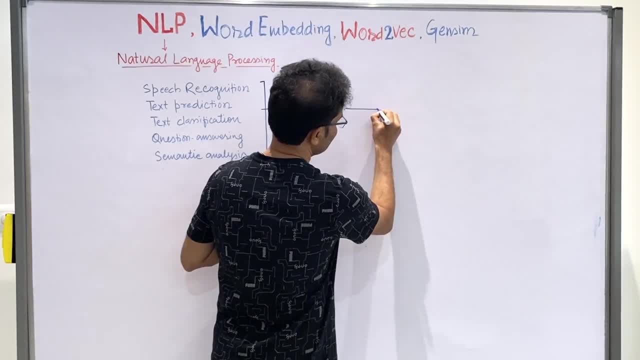 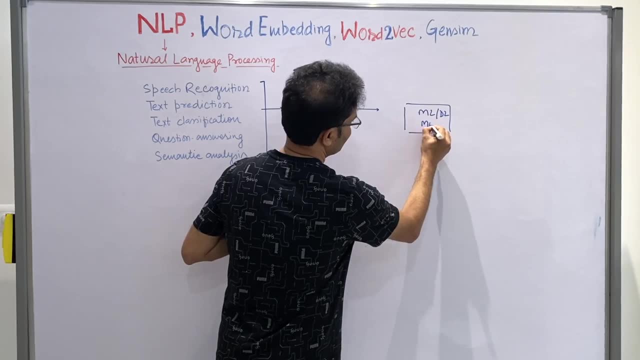 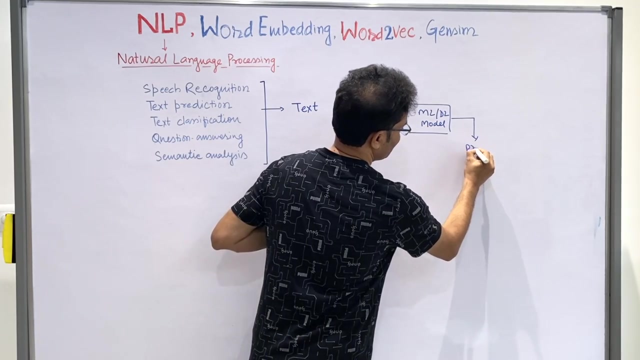 is the text, and then you put this text into some machine learning model or deep learning model. that will take the text input And they will take the text input. And they will take the text input And they will give the output as a predictions or whatever you want to achieve. 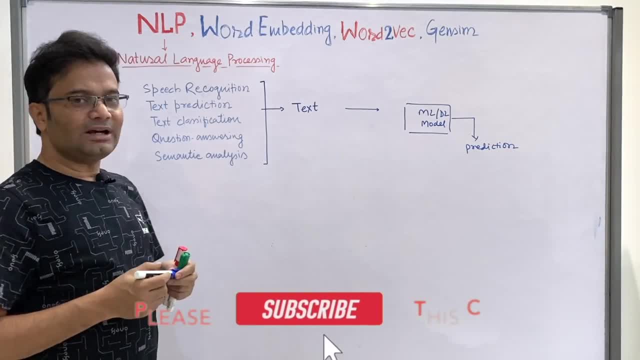 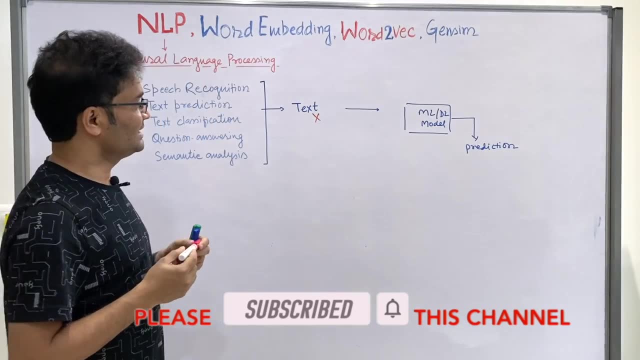 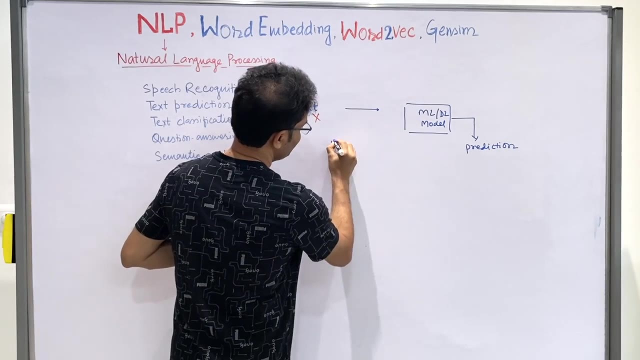 But we know the machine learning model can only understand the numbers. they cannot understand your text. So you cannot pass as a text into the machine learning model. So for that what you have to do means some system should be there where you can pass. 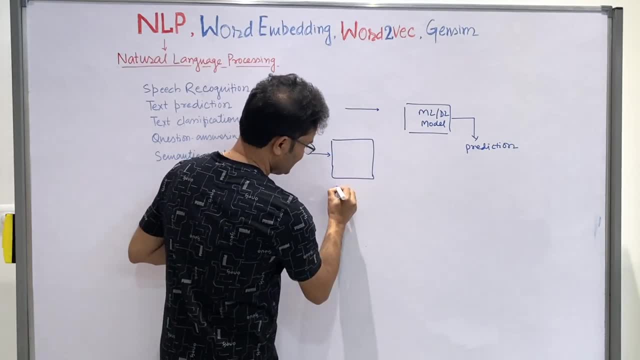 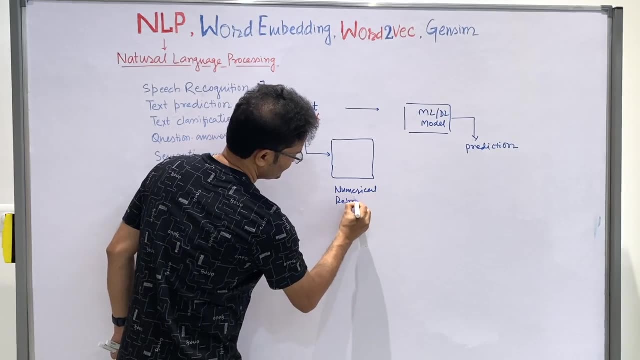 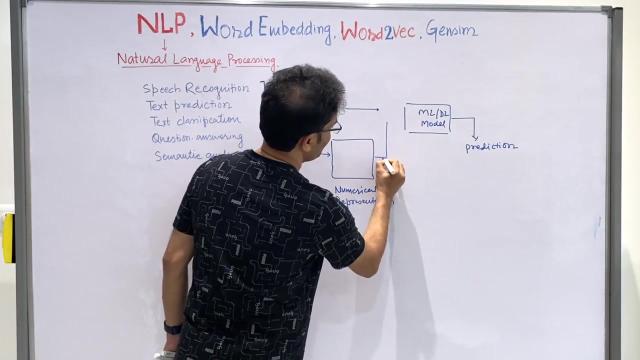 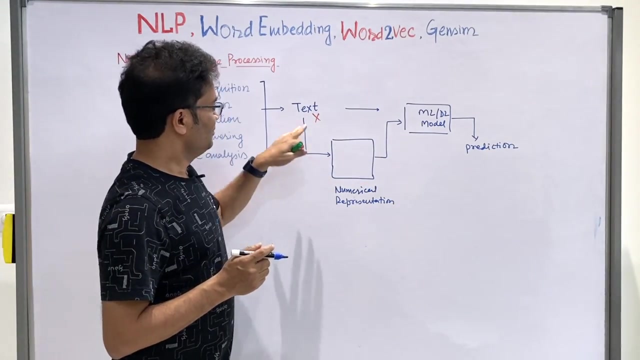 this text, So that is the NLP, And this system can convert your text into the numerical representation and then that numerical representation you can pass into the machine learning model, That model. then this model will work as it is used to be work when you passing the numerical. 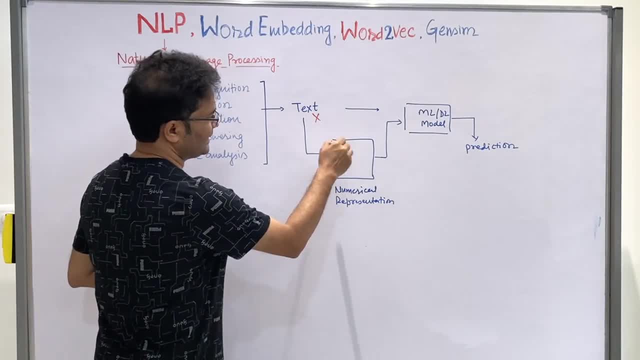 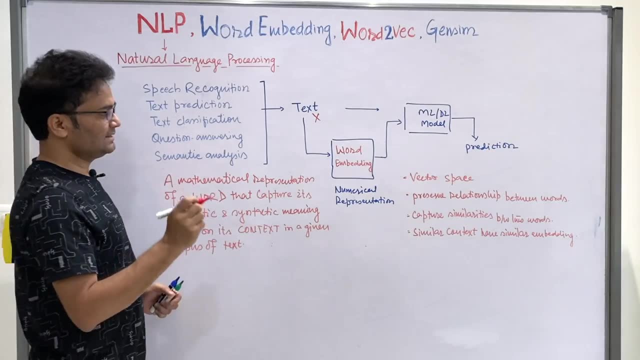 representations. So the important thing, what is that thing? that we convert your text into the machine learning model. So the important thing, what is that thing? that we convert your text into the, into the numerical representation, And that system is called the word embedding. 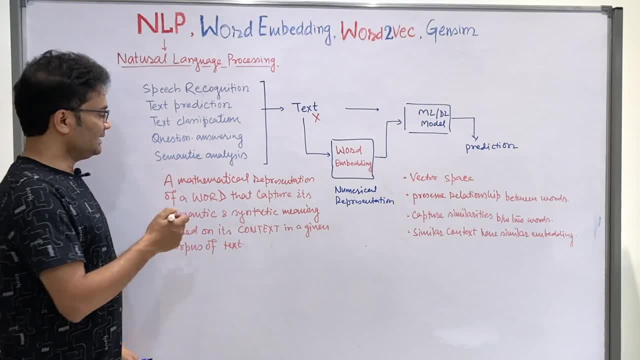 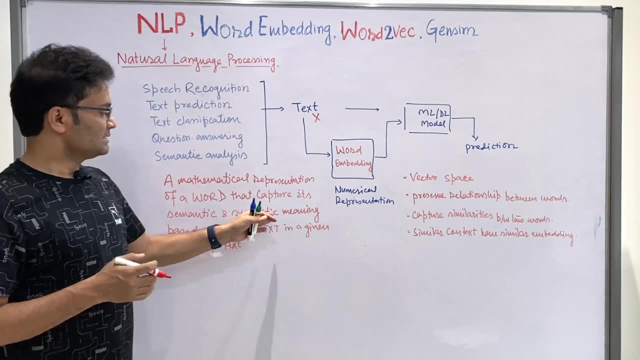 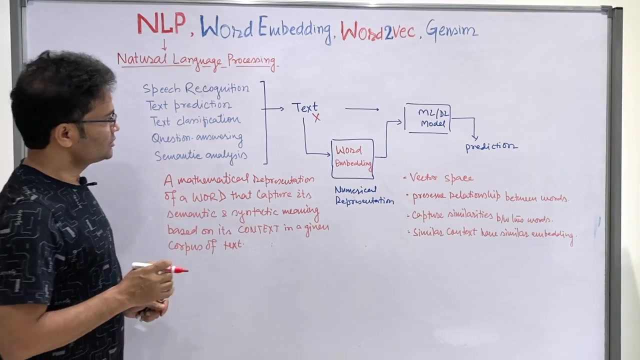 So what is word embedding? Actually, that is the mathematical representations of the word. that captures is the semantic and the syntactic meaning of a word in the given of the corpus and given the context. So suppose, if you give the one word apple, orange, man, king, queen, 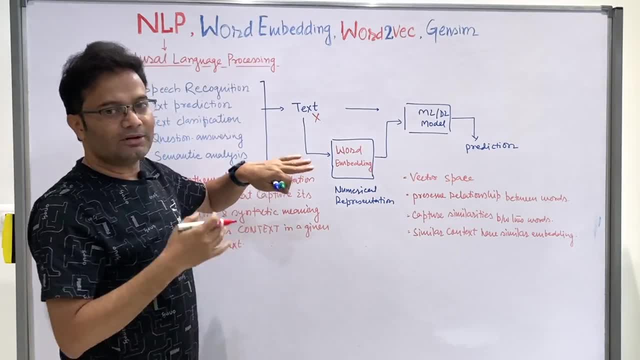 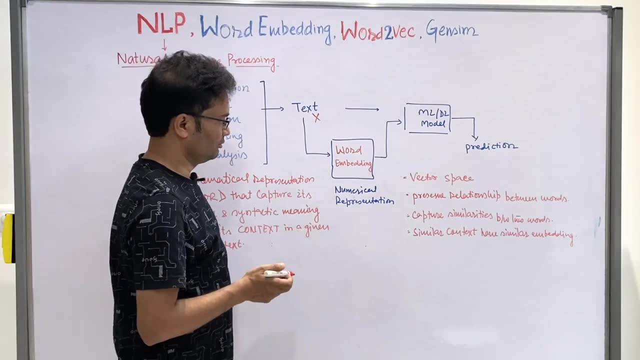 Then if you give the one word apple, orange man, king, queen, Then if you give the one word apple, orange man, king, queen, queen, they will convert into the numerical format and that is actually a vector that I will show you in the code also and I will explain you in detail also. 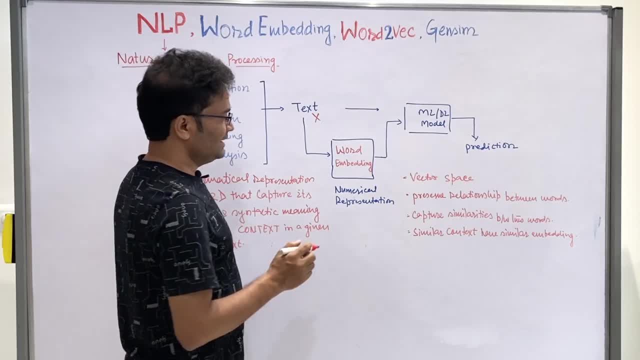 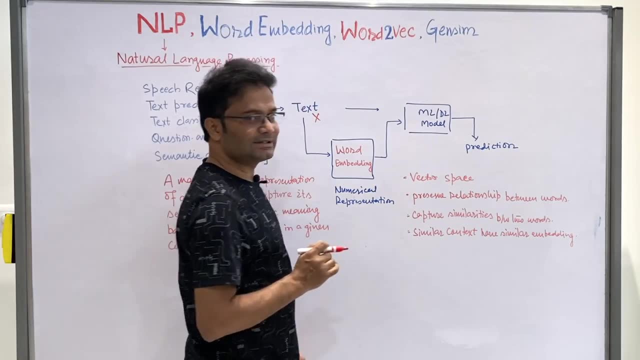 So if you see the what is the word embedding? word embedding is a vector space that contain the meaning of a word, depend upon the given context. it preserve the relationship between the two words. So if there are the many words in the corpus, what is the connection of the one word to? 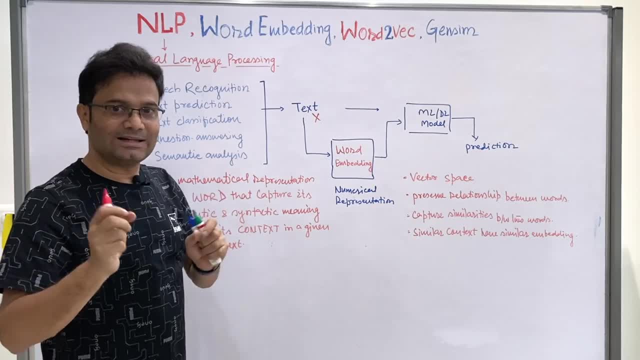 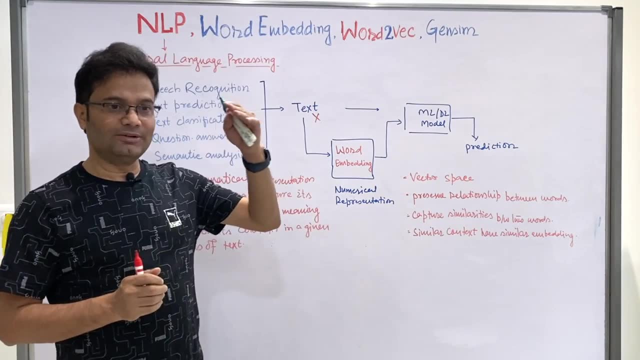 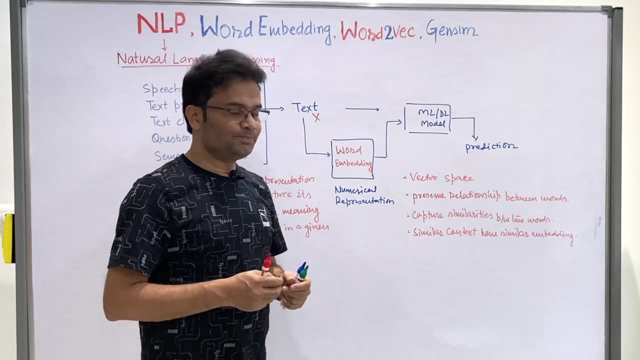 the another word that maintain the relationship. what is the connection of those things that that can be preserved by the word embedding right, the capture, the similarities? Suppose if you given the one word and find out what are the similar words in this corpus, that also you can find out. 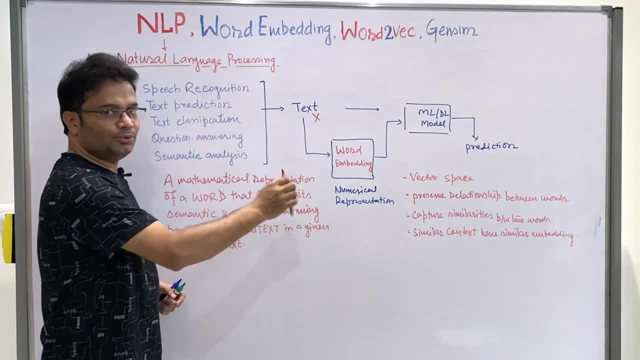 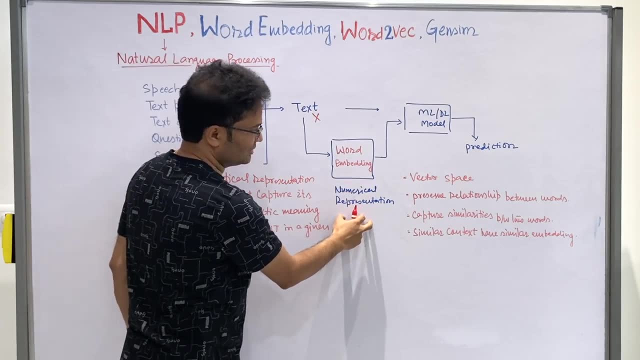 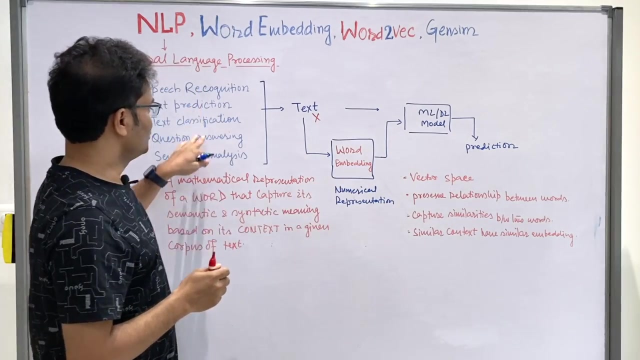 So this is very important if you want to do anything in the NLP, because it will convert, embedding, will convert the text into the numerical representation. Then you can use. You can use numerical interpretation for the any inside any model and you can find out all the execute one, any of the use case right. 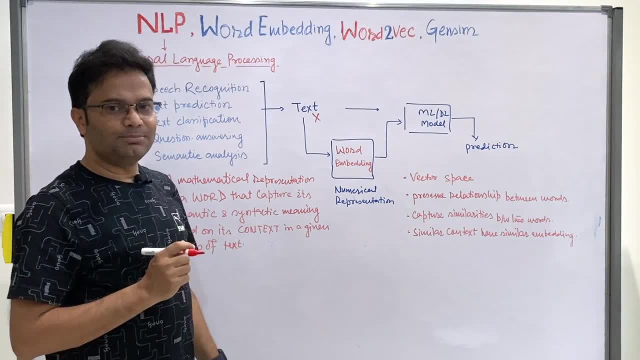 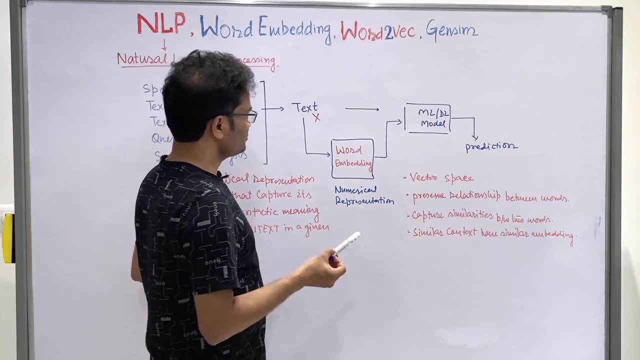 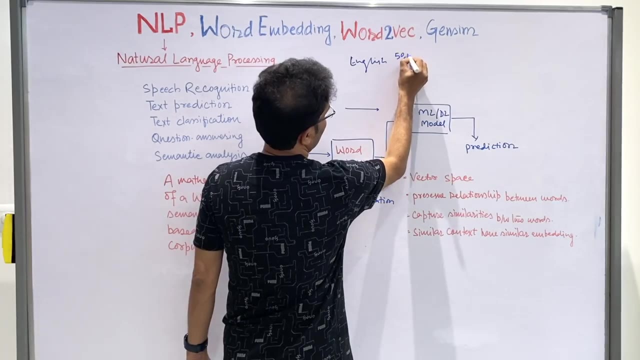 So why the word embedding? it is very simple. So why you cannot make give one ID for the each word. So suppose, if you see the English dictionary, so suppose I have the 50,000 words in the 50,000 words in the dictionary. 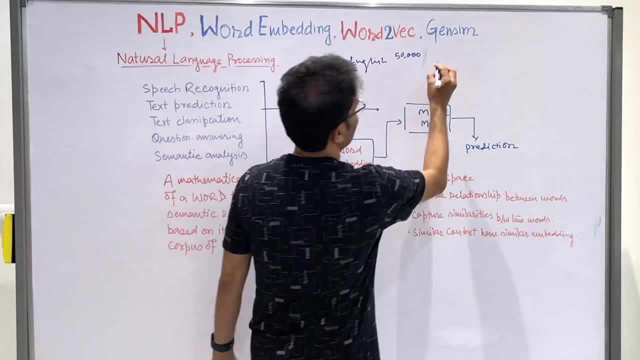 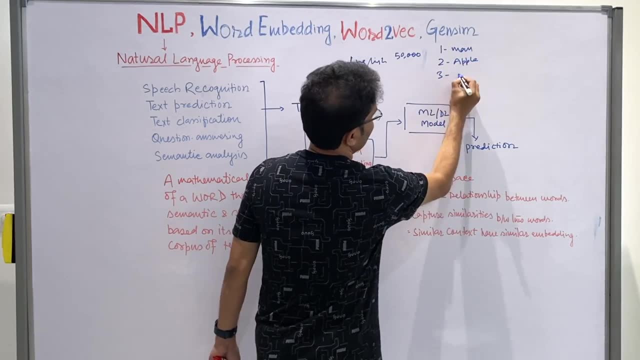 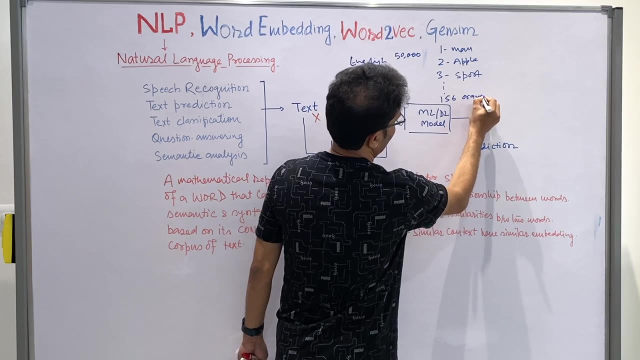 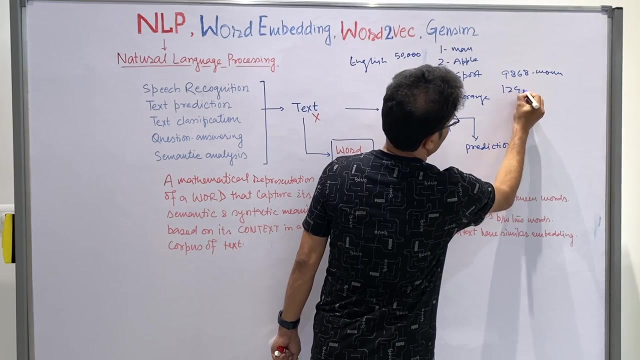 So you can give the number. So suppose I do give the one number, man two number, apple three number, anything sports. Suppose 156 is the orange, 9860 is a woman, 10950 is the king. It will not work. 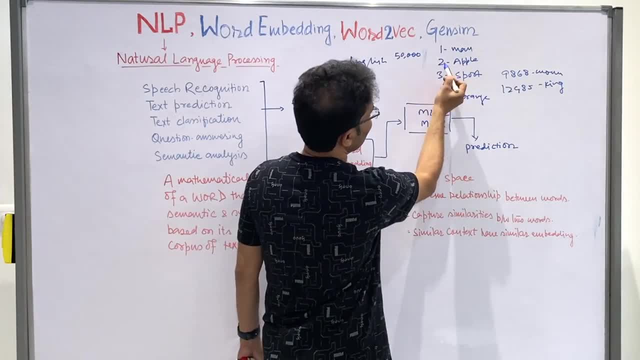 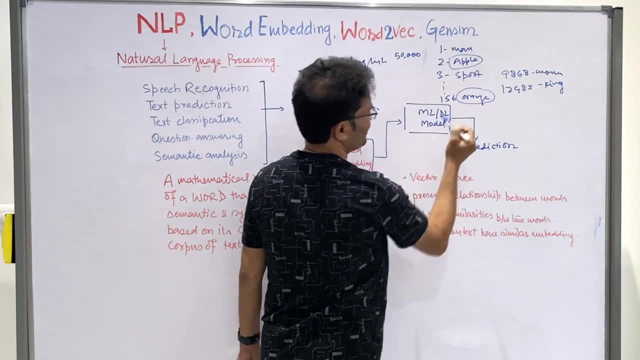 Why it will not work? Because then if you see the apple number, you have given two and the orange you have given that 156, but you know, some connection is there between the apple and orange, but numbers are the two, five. 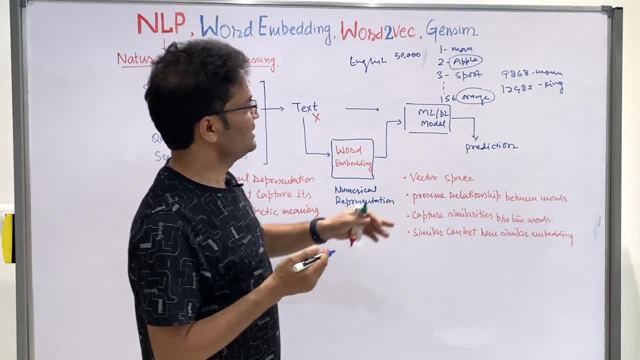 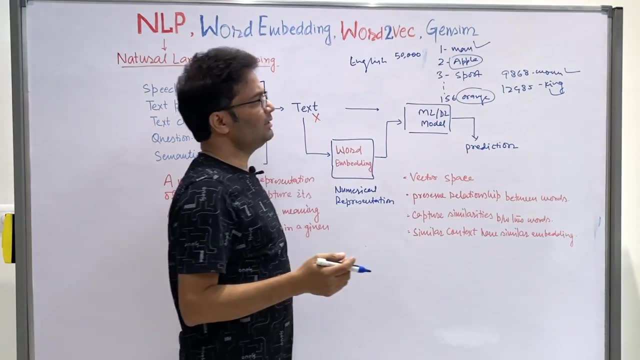 You cannot make any meaning of that right. If you do the similarities, there is no similarity If you talk about the numbers, the same way. if you see the main king- women- these are the women being, but the ID is very different. 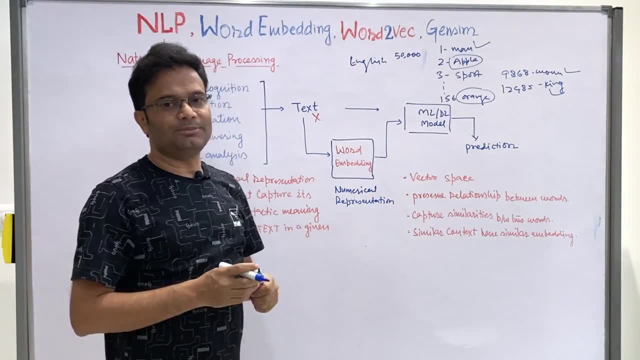 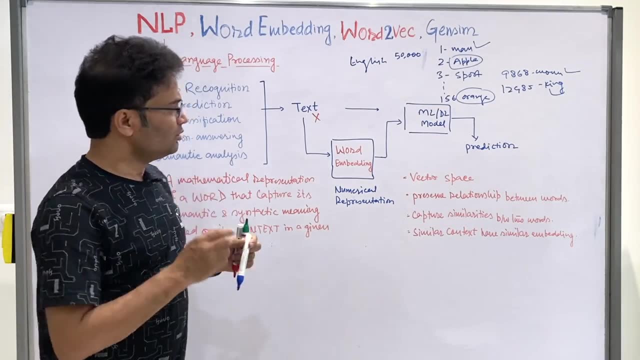 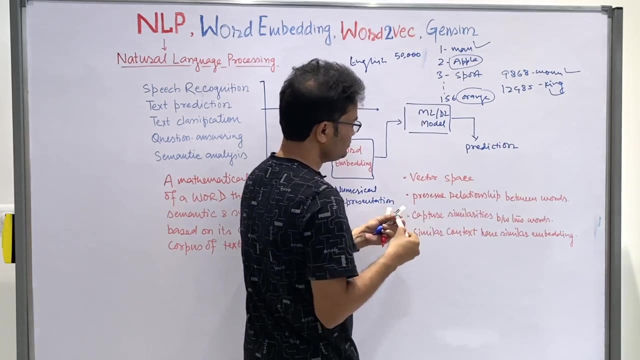 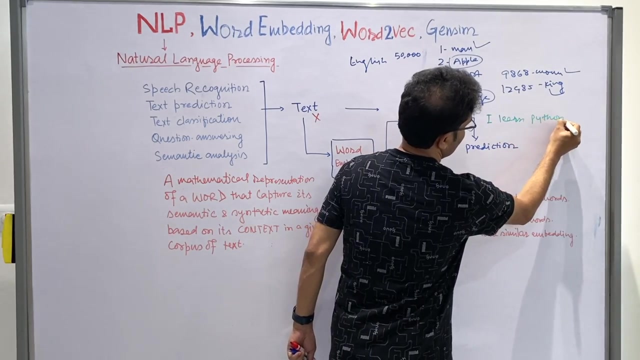 So this thing would be not work. So that's why this word embedding come in the picture that they can reserve, Okay, Or they can preserve the meaning of a pod article for the given context. So let me give one more example. So if you see the, this sentence, if you see the, I learn Python. and another sentence today. 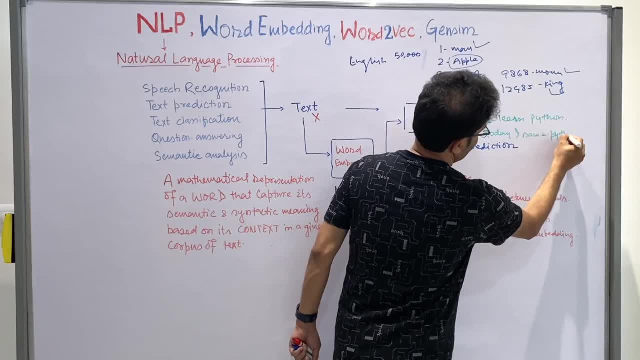 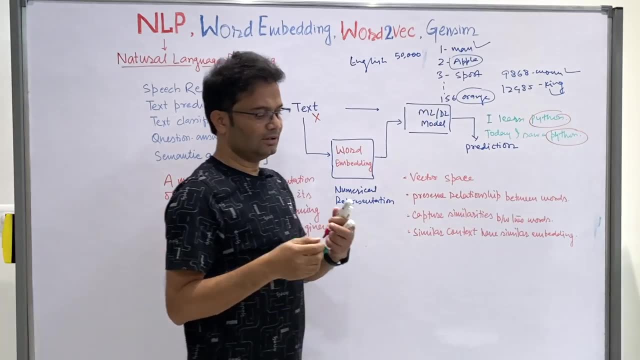 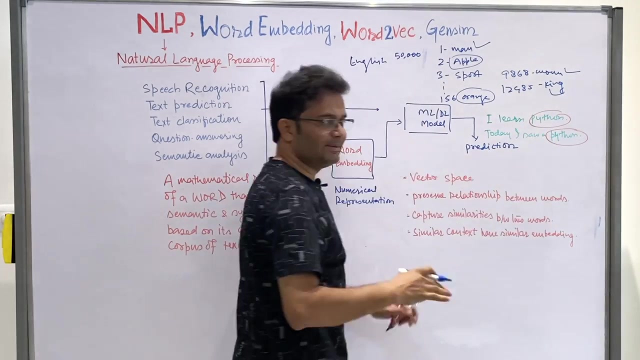 I saw a Python Python. What is the same here. Here is the also Python. Here is the also Python, but the meaning is different, right One, this sentence Python means the programming language, and this sentence Python is a very big snack, right. 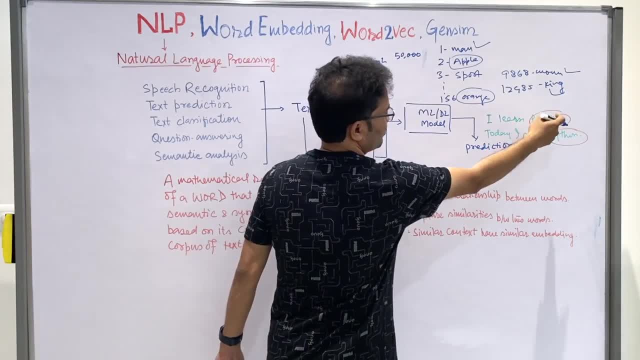 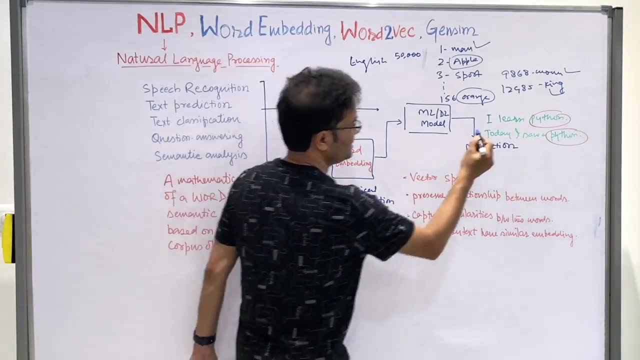 So in this case, if you give the ranking for the number one, two, three, four, that system will not understand what you are saying. But if you make the the word embedding, for this Python you will get the different representation and for this Python it will give the different representation. 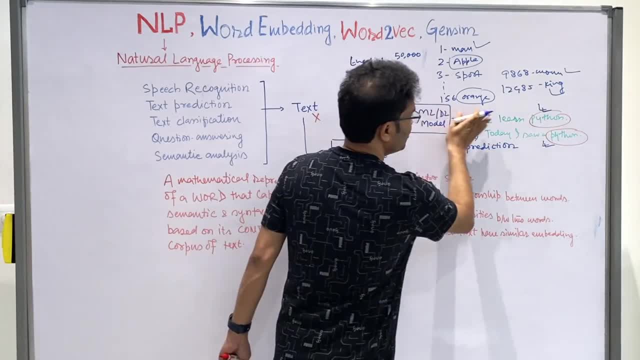 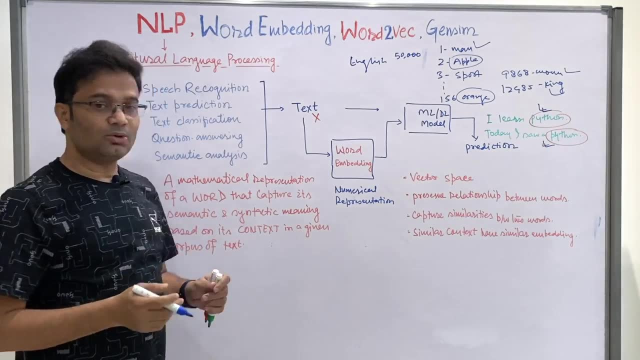 Because they will consider the whole corpus to making the embedding for particular words. So that's why word embedding is very important. We will see in the code why it is important. Now, if you see there are the many different kinds of the embedding right. 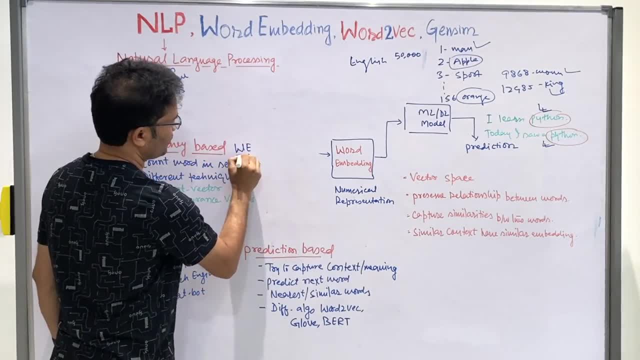 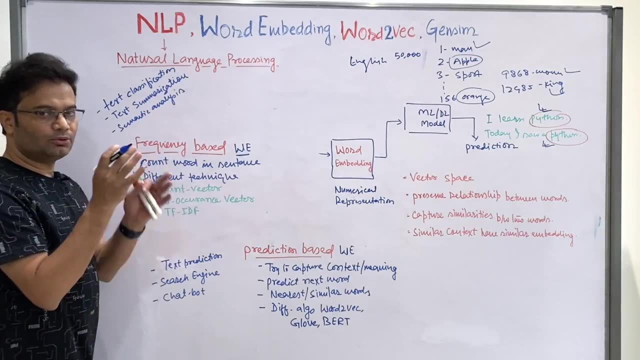 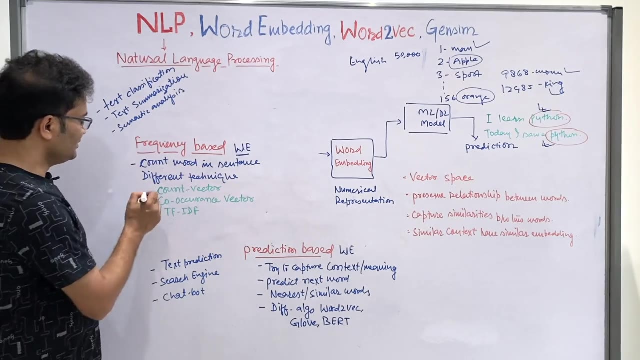 One is the frequency based word embedding and second is the prediction based word embedding. So in the in the frequency based that we count the particular word in a given sentence or in the different document to find out the test classifications right. So these are the different techniques by which you can do the frequency based word embedding. 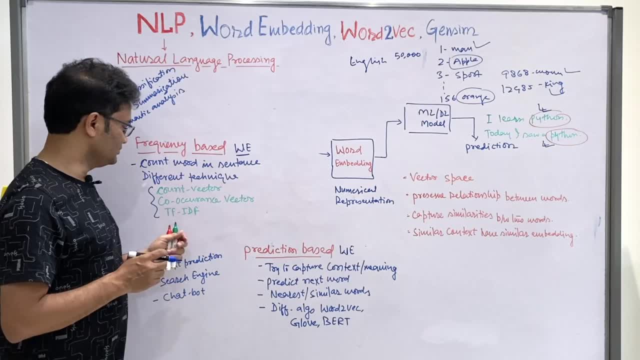 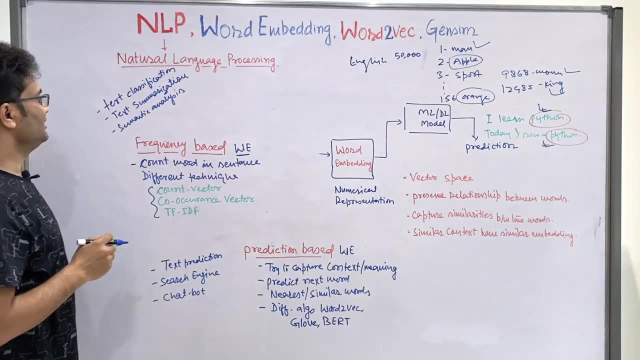 One is the counter vector. second is the co-occurrence vector, third is the TF-IDF and the main use case of the frequency based word embedding is the test classification text, some variations and the semantic analysis. If you see the, these are the things main use case for this one and if you see the prediction, 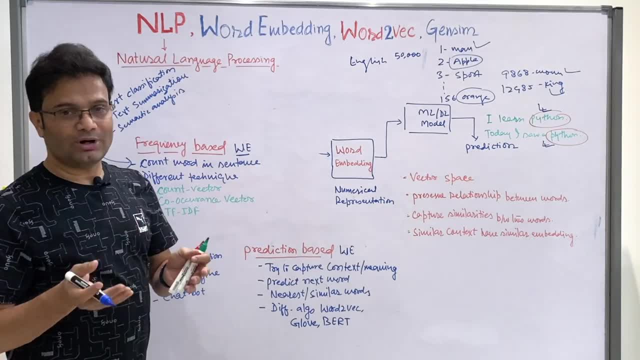 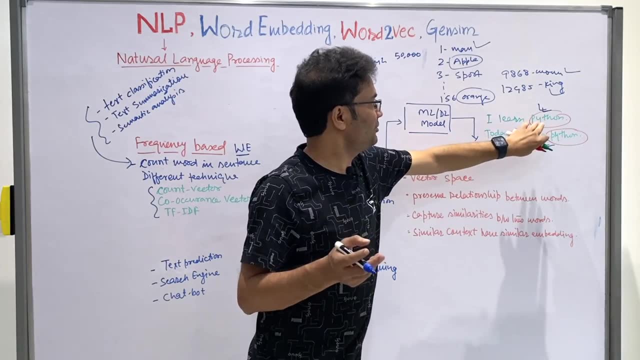 based word embedding, If you try to capture the context, means if you give on the sentence here, if you give on the sentence from this sentence. they want to know what is the purpose for the Python here and what is the purpose for the Python here. 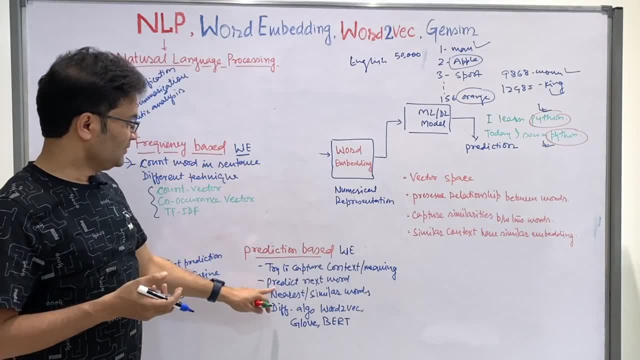 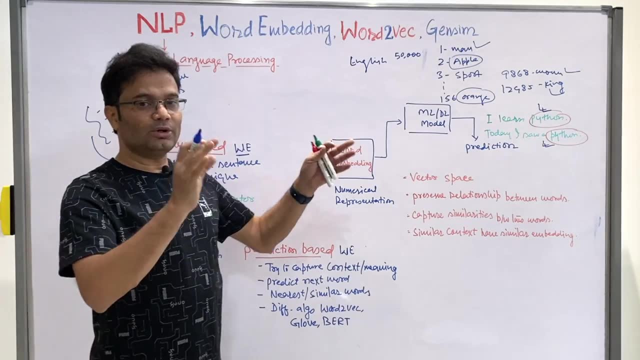 So they are trying to capture the context. what is the meaning of that and the predict, the next word, as I explained earlier, and what is the similarities and the similar words? So if I give on the one corpus and among that corpus, if I say one word, suppose a man or 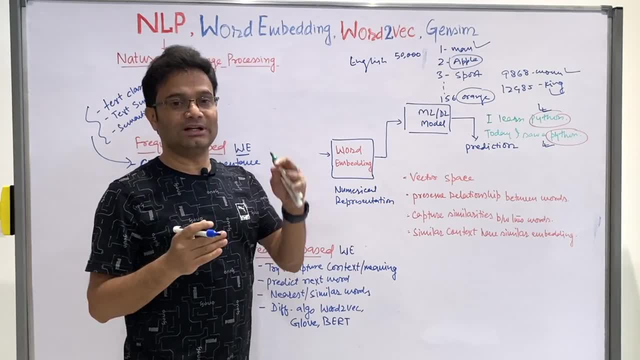 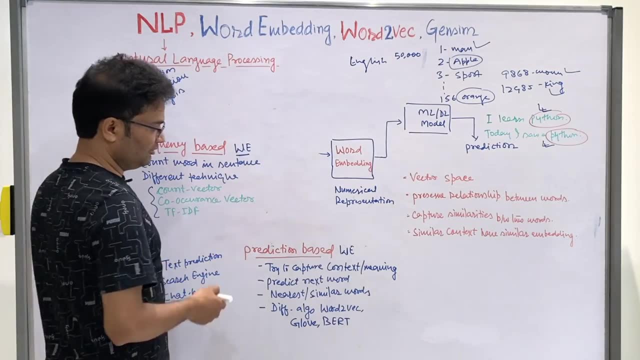 the king. What are the different similarities Words are there in that corpus? that also we can find out for the prediction based. So there are the many algorithms by which you can do the prediction based things, And one is the very famous word2vec that we are going to see below and the word but next. 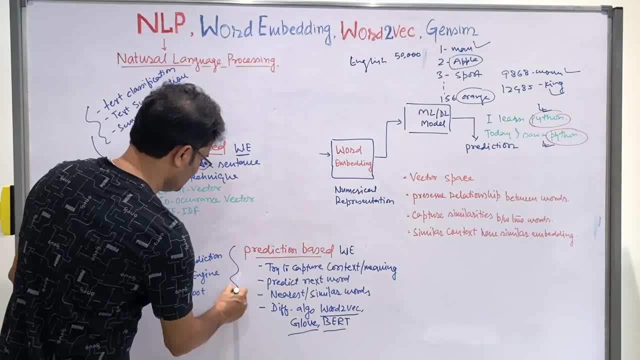 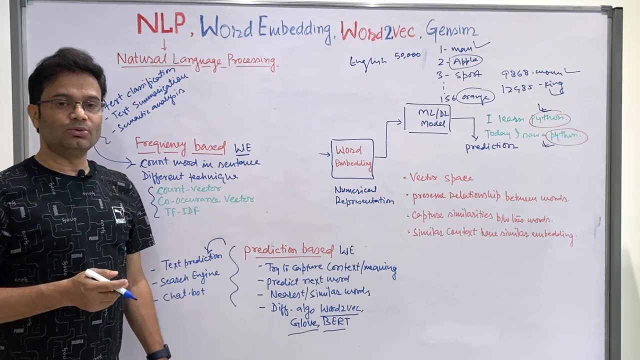 video I'm going to make on the word, You can see that And these are the use case for the prediction based word embedding text prediction search engine. So if you search in the Google right, if you give on some sentence, they can find out in. 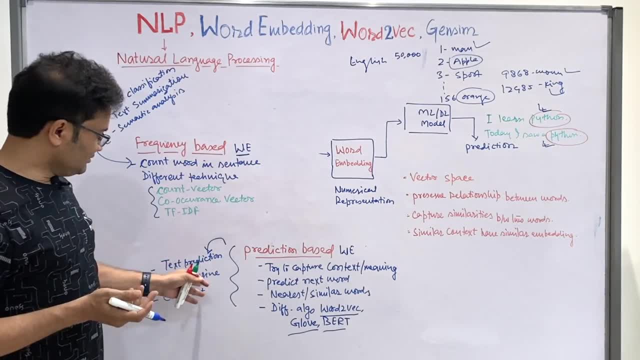 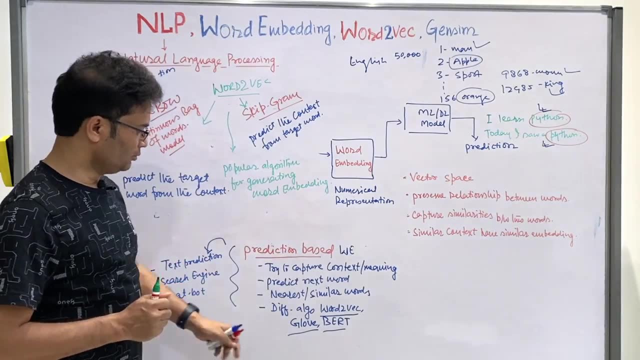 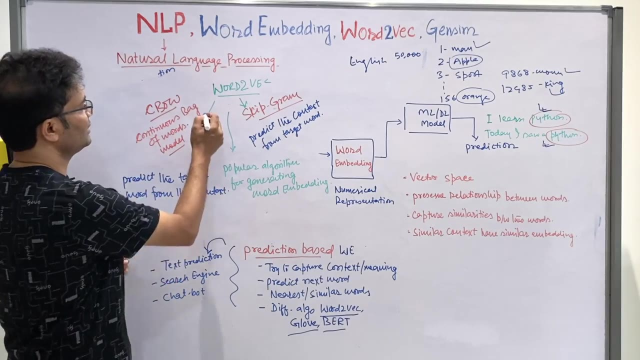 which context. you're asking something right, So that search engines have. we used the prediction based word embedding, right? So if you see the prediction based word embedding, we have the different algorithm, word2vec. So if you see here the word2vec, they have the different models inside the word2vec. 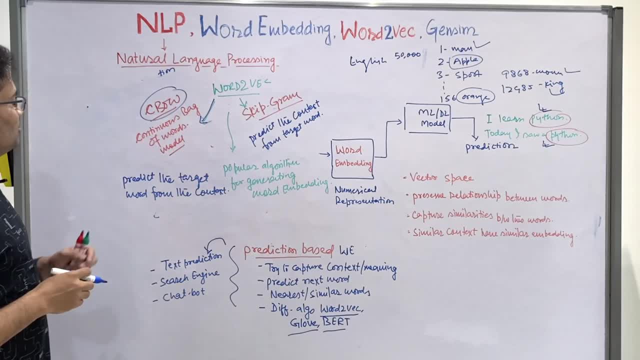 One important model is called the CBOB- continuous bag of the word model, and another is the skipgram, So actually the CBOB. So what did you do that? If you give some syntax, syntax or the text, they will predict the. what is the target word? 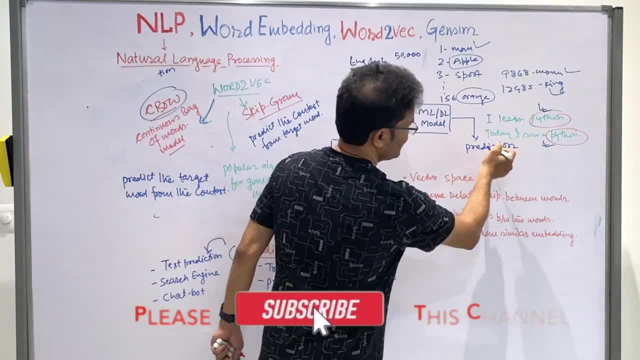 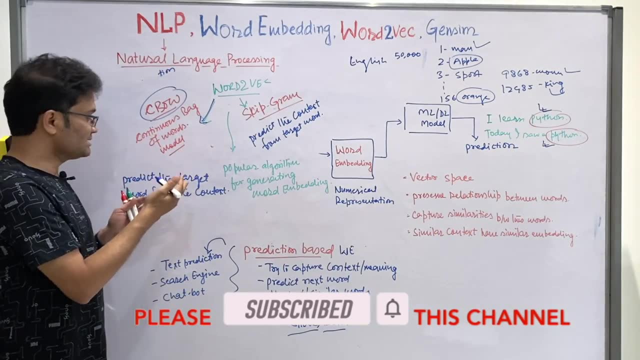 from the given context. So if you see in this sentence, they try to find out what is the target words. If you can see here, Python is the target words, right, So they will try to find out the what is the the target words in the given corpus. 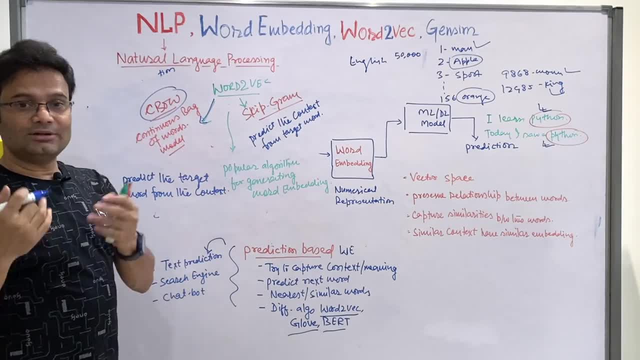 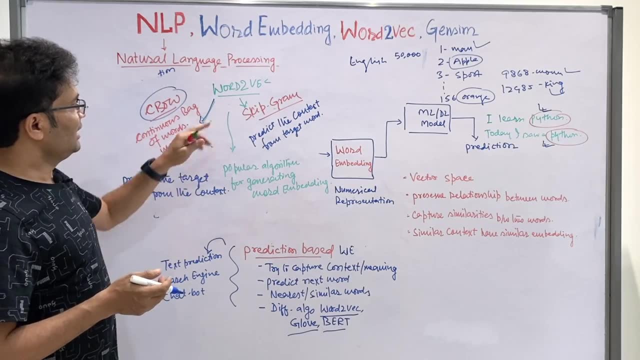 In the appogit. if you see the skipgram, they will find out the different words from the target words. So we use a different for use case, we use the different models And, as you, I said that word2vec is the proper algorithm who generate the word embeddings. 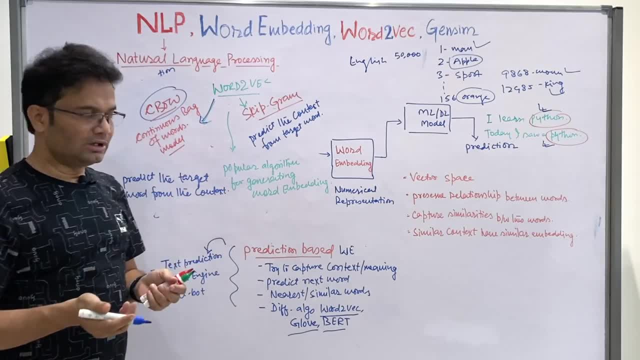 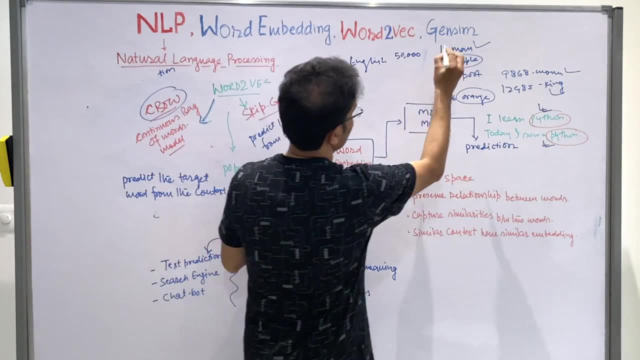 right. So the word2vec algorithm, we will generate the word embedding for the given corpus that we will see in the code. So the and the one is the. this one, the genSIMS. genSIMS actually is the very famous. 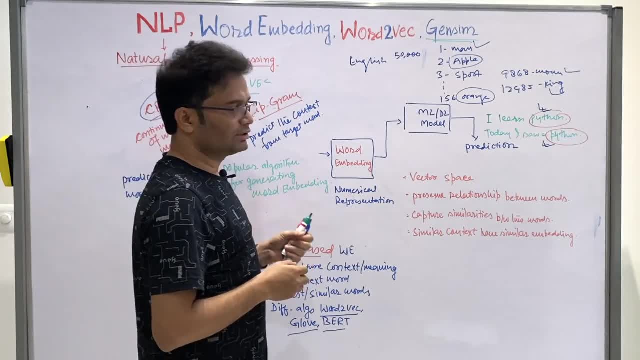 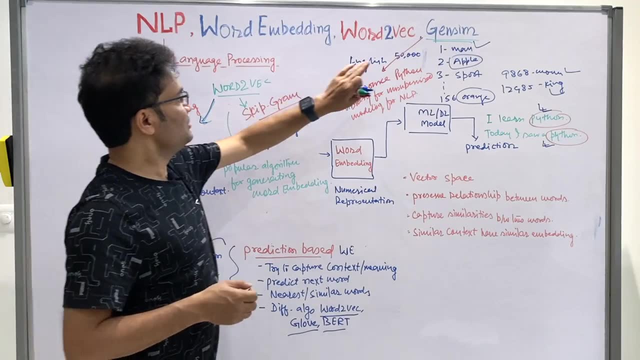 Python libraries. Using the genSIMS, we will execute all the algorithms, So we will use the word2vec And we will generate the word embeddings. So, as I said that, genSIMS is the very famous open source Python library for the unsupervised. 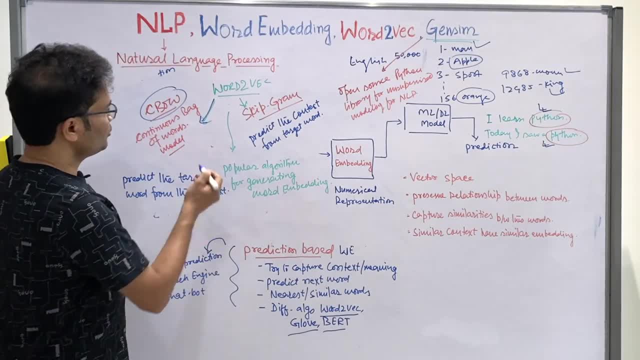 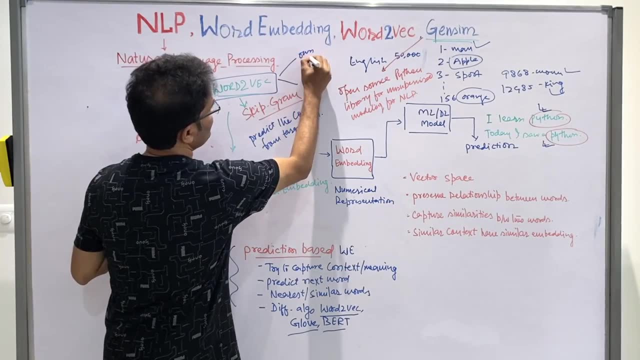 modeling for the NLP, So that you are going to use that, And also when you go to the use the word2vec. so we have the two options to use that. Either you can use our own corpus. we will give our own corpus and do all the operations. 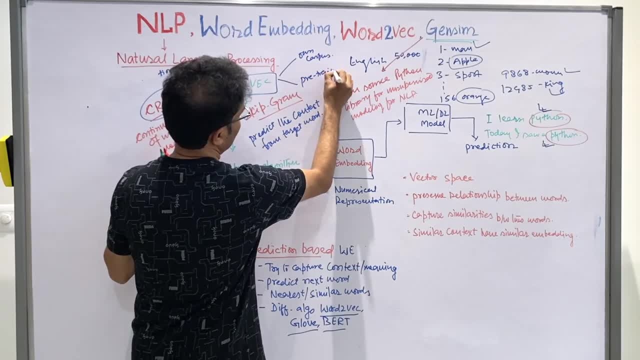 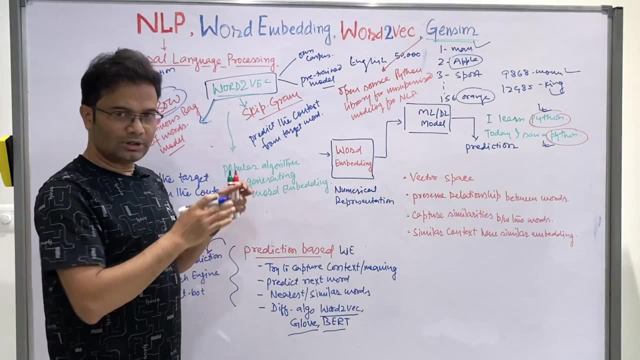 or we can use some pre-trained model also, And then we can do all the operations. So everything you are going to see in the code. So again I will say: you complete whatever I am going to show in the code. you repeat the same thing. 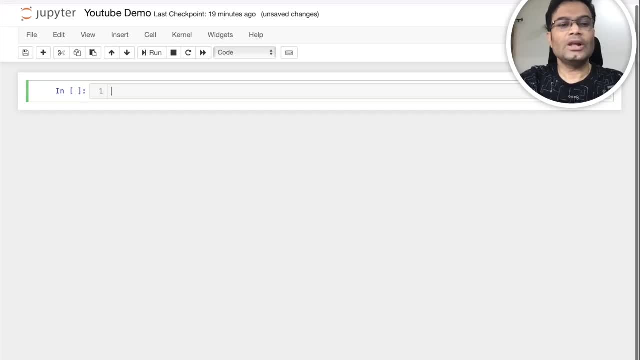 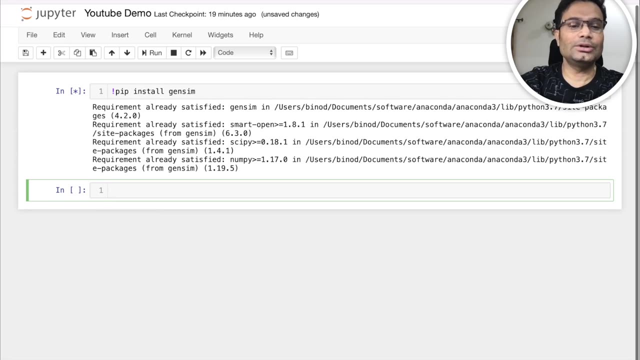 So you will have the good understanding on the complete Python code. First and foremost, we need our genSIMS library, So we have to install it. I have already done So. it will not execute here, But in your case you have to do that. 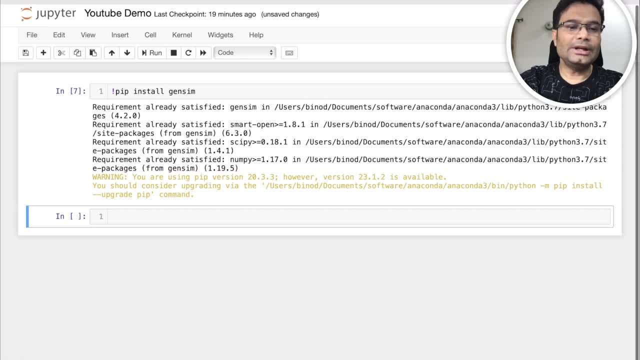 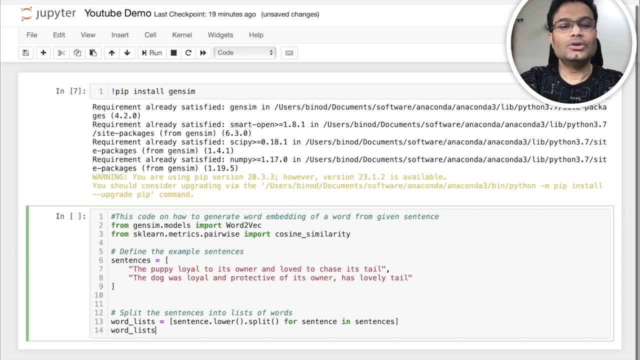 What I will do for this example, for this demo. So take one, two simple syntax, right this corpus and then find out how to create the embeddings. So for that, what I have done, that we create one model with the help of the genSIMS. 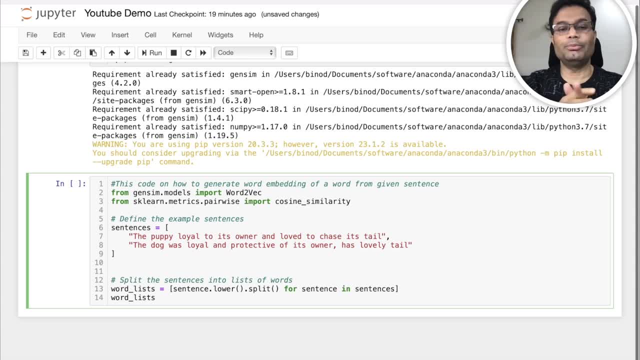 And also we took the cosine similarity that we can use to match the similarity whether one word is matching with the other words or so not. So I have taken the two sentence here right, the single sentence for the dog and puppy. But you know, in the NLP you have to pass the words inside the model. 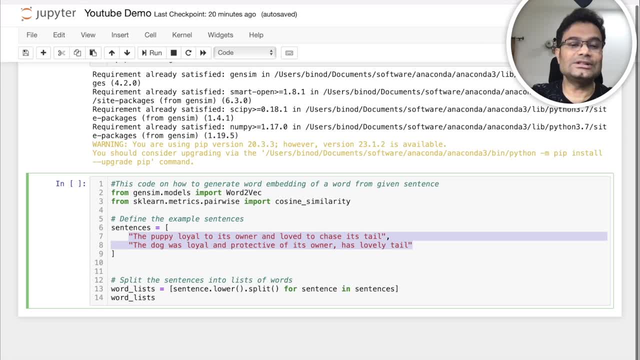 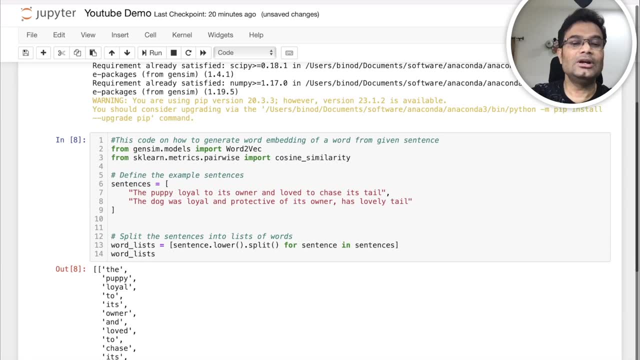 You should not pass the syntax right. So that's why I convert this sentence. I took the each word, Make it, split into the words and make one list, the word list. So if you run it you can see all the words of this sentence has been broken down into. 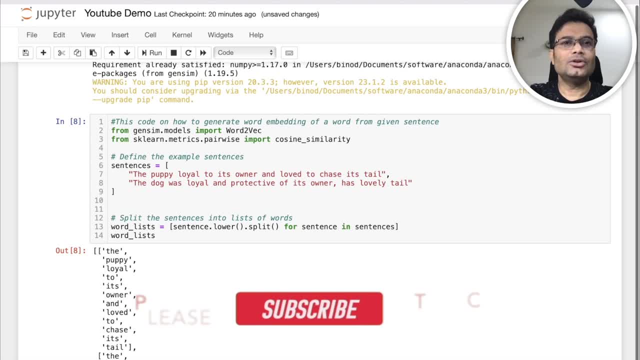 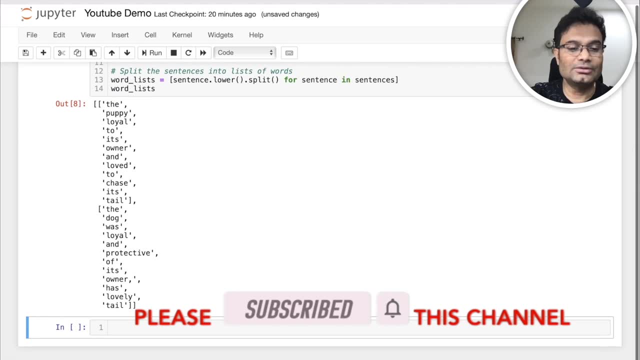 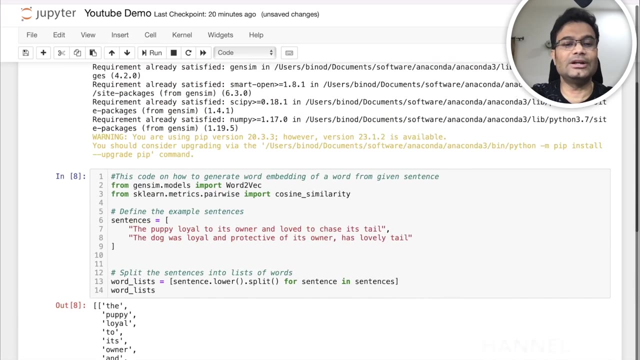 the words. Once you do that, then now we can see the what is the embeddings value. So now we can find out the each words: what is the word embedding? So let me paste this code Here. what I did? I passed these words into the word2vec model that we have created, right. 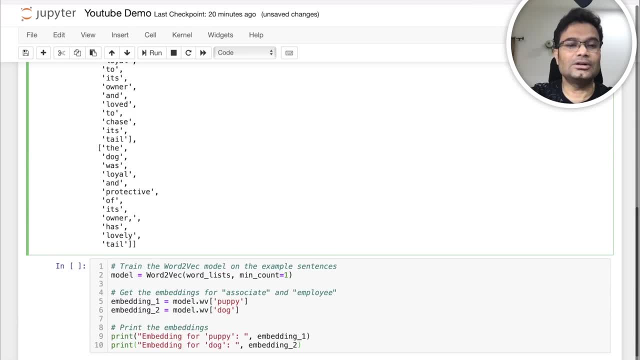 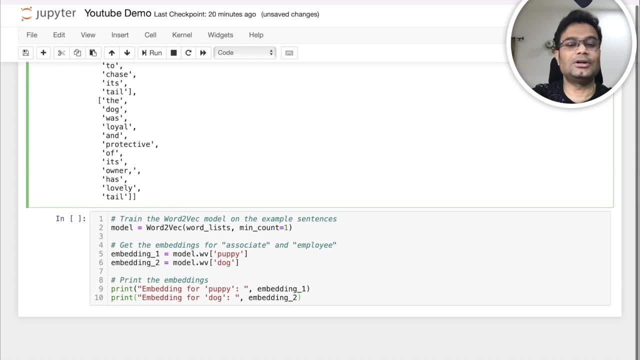 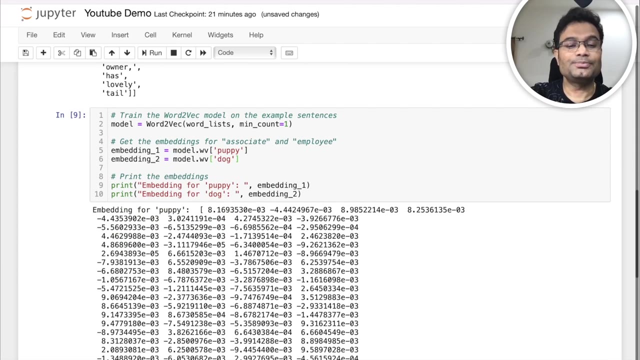 now here, right, And then I pass this list of the words and then we can check what is the puppy embedding and what is the dog embedding. So very nice If you see here, this is the you know the word: embedding vectors, space vectors for. 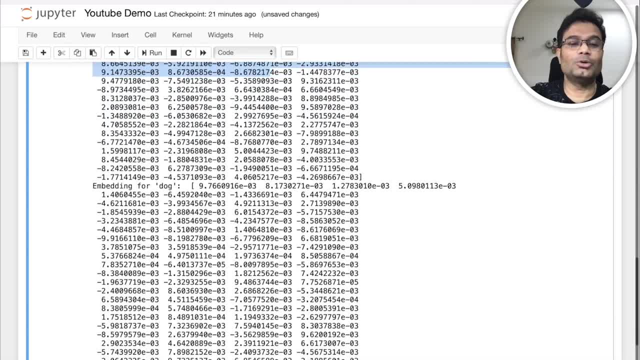 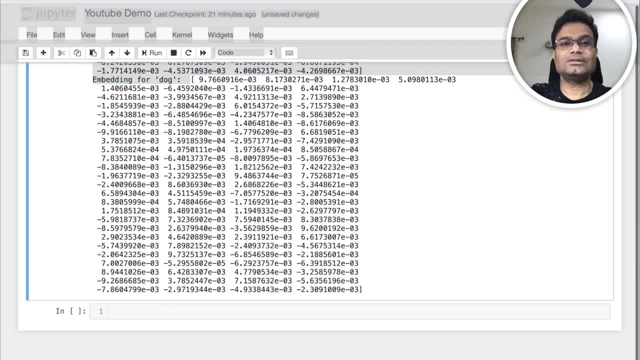 the puppy. See, use data that have taken the almost a hundred dimensions right. So actually the corpus is not strong, that is a hundred things. But if you see the, if you take the bigger data, you can see the bigger corpus, the dimension. 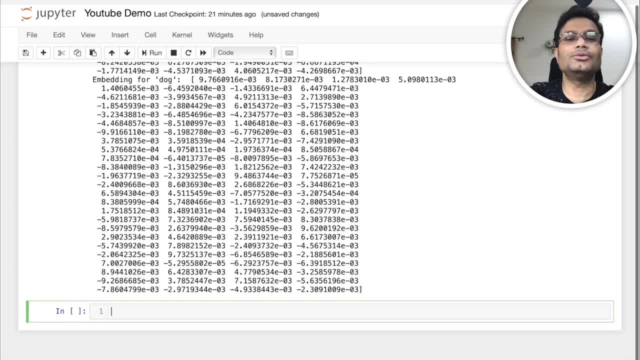 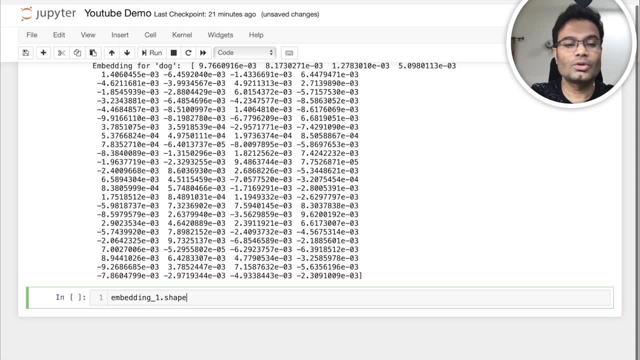 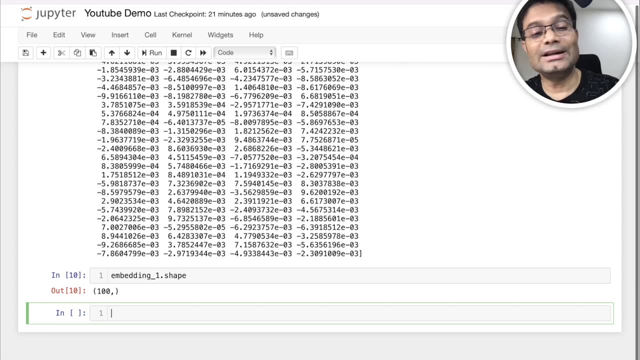 is going to increase. Let me see that, how much dimensions we have. So if you see what is the first one embedding one, go and see what is the size of this. So it is showing the hundred one. So that's why it is able to preserve the context and the meaning. 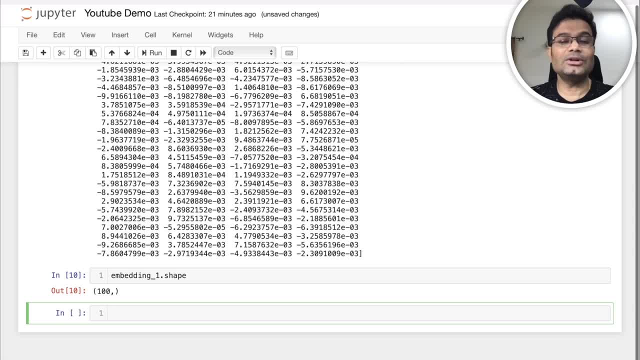 They took all the properties of particular word from the corpus. That's what is able to maintain everything right, So that's why it is able to preserve the context and the meaning. They took all the properties of particular word from the corpus. Now, once you do that, now what I will do, I will. I says that I took the embedding for 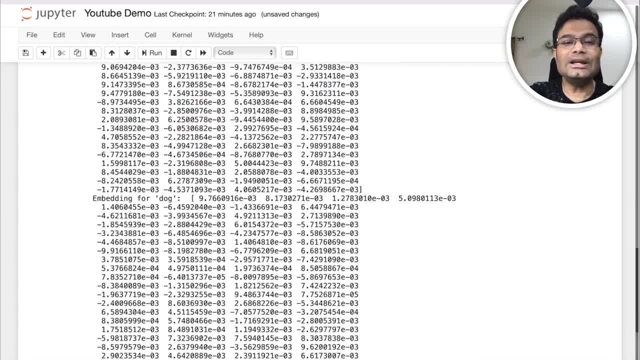 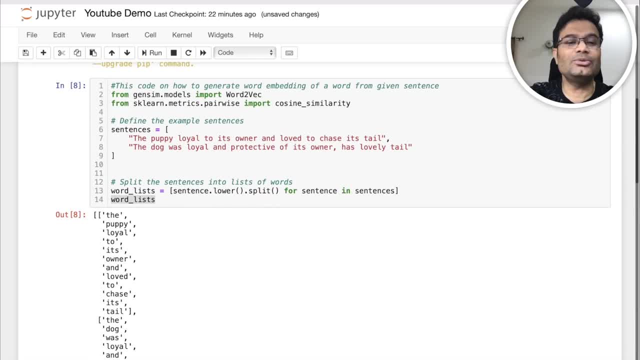 the both right. I took the embedding for the puppy and dog. Let me see: is any similarities between these two embeddings, between these two words, puppy and dog, because I have taken the sentence in such a way that it looks both should be. 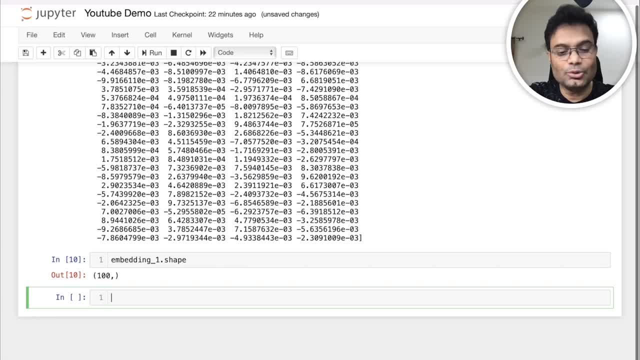 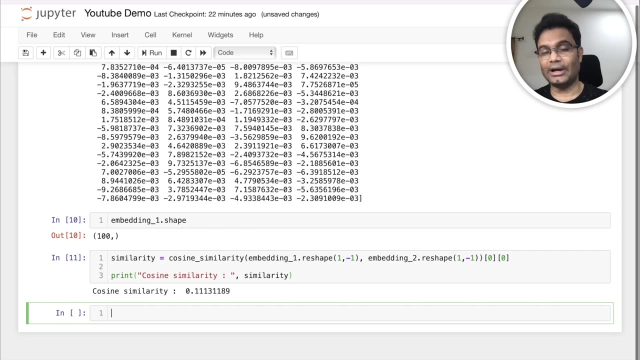 the same right. So I pass this, both embedding embedding one and embedding two inside the cosine similarity methods. See how much equalities are there. If you see it is the 0.11, means cosine similarities varies, vary from one to the minus one, minus. 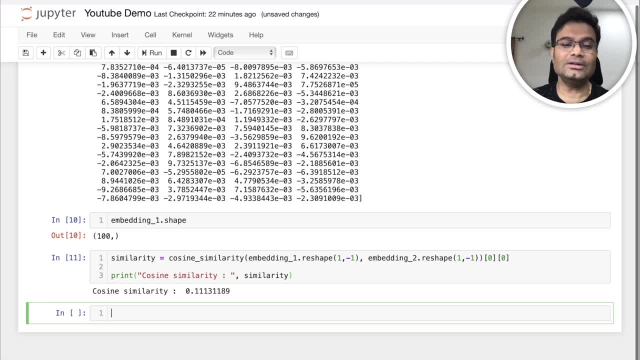 one to the one minus one is nothing matching. One is the high matching and it is showing the almost 10% is matching because our corpus is not too high. So that's why it is not showing, As I showed in the video, that you can use the word to back with retrained data also. 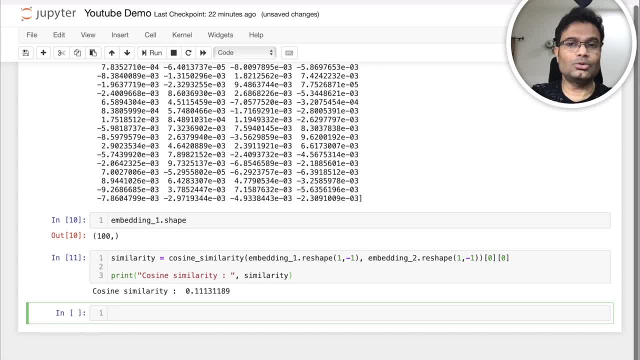 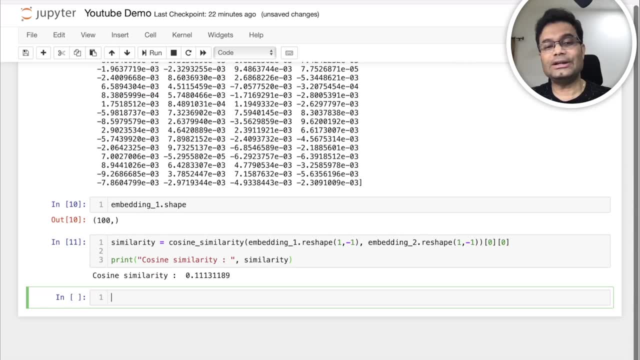 and with our corpus data also. So what the the code I showed, This is what I showed. This is our data in the corpus, right, This is our data. But now Google and their team has made one very good corpus, almost a very big millions. 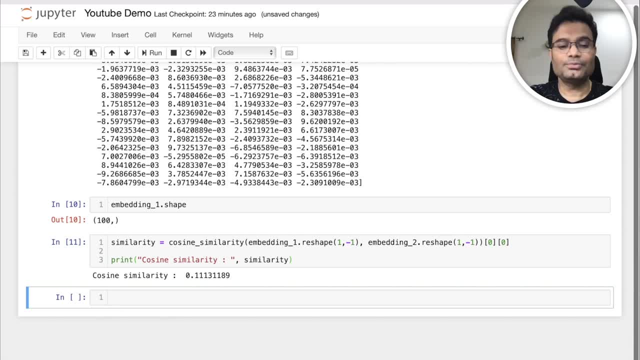 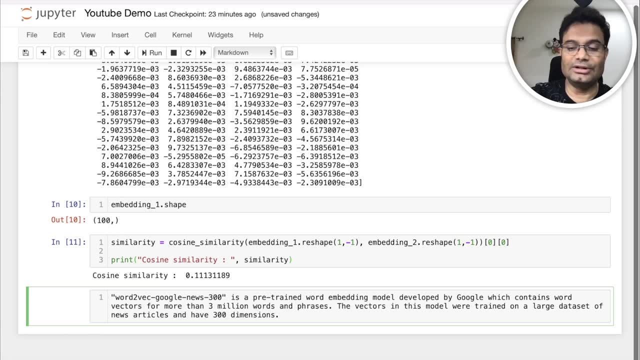 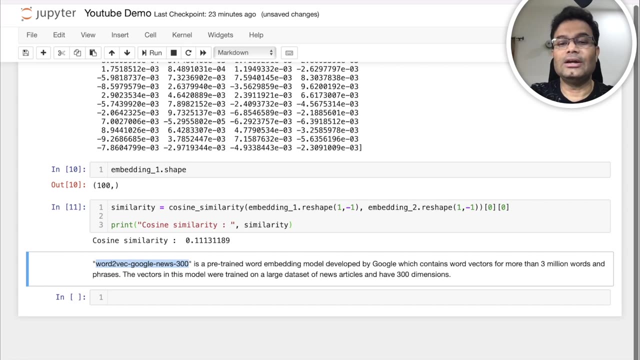 of data. they have taken that So that I'm going to use here and then you can see everything over there, almost most of data over there, So it's very easy to generate anything. So that name is the word to back Google news 300, it's a pre-trained model and that they 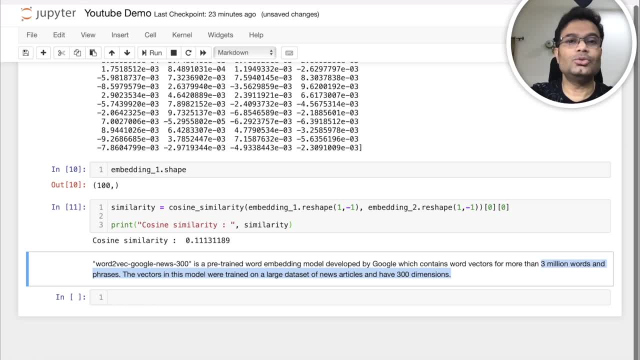 have the three millions words and the pages right. So we are going to use this print data model, a pre-trained model. So how, how you can use that. So it's very easy. So you go. we have already installed the gen sims. 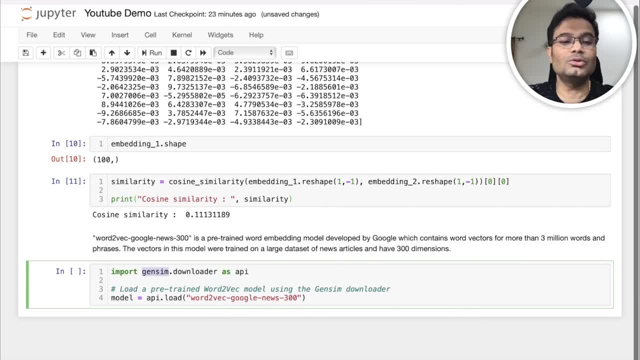 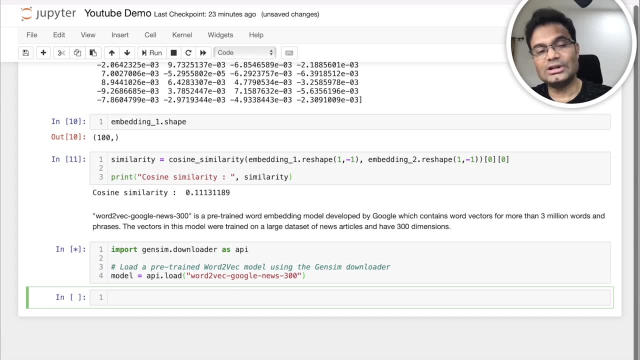 So use the downloader API and see which model you want to download. So I want to download this pre-trained model and just run that. It will take some time because they have the use size, but just you have to wait for that right. So if you don't, if you want to start from the pre-training, then these two lines of: 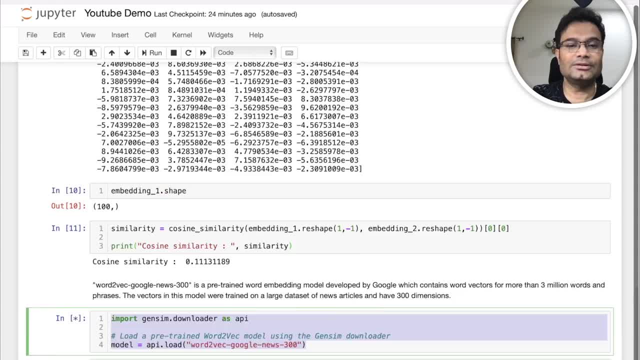 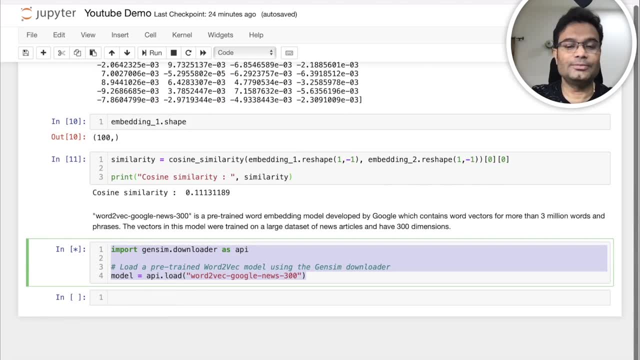 code is sufficient, No need to do anything. what I have showed you over here, right? So I showed using my own corpus text, but here you can use the pre-trained model. Once this execution done, you can see. and just I want to see what is the word embedding? 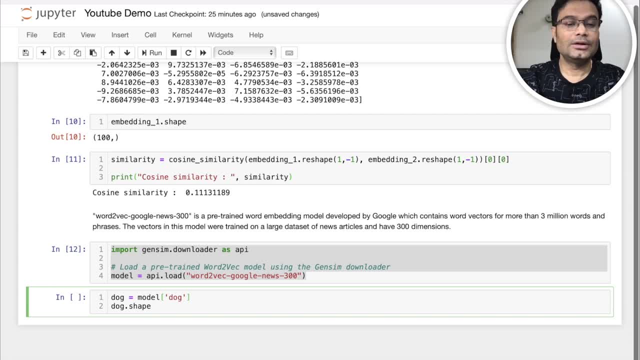 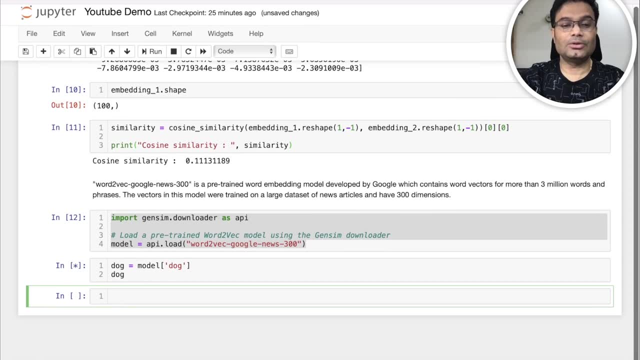 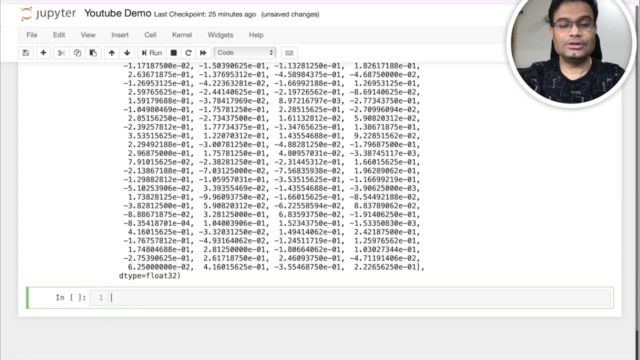 of for the dog, right, according to this corpus, And if you see just dog, So they generated, Okay, Generate this much big corpus, the word embedding for the dog, see, And if you see the, how many dimensions are there? 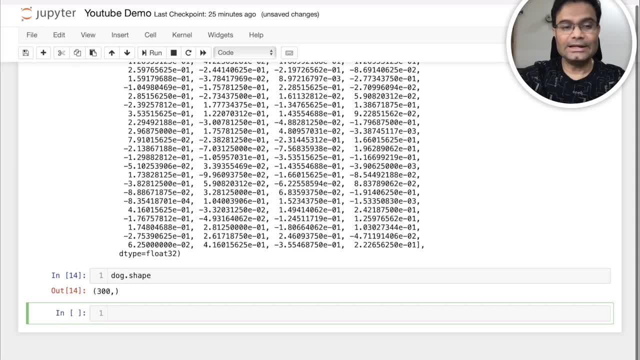 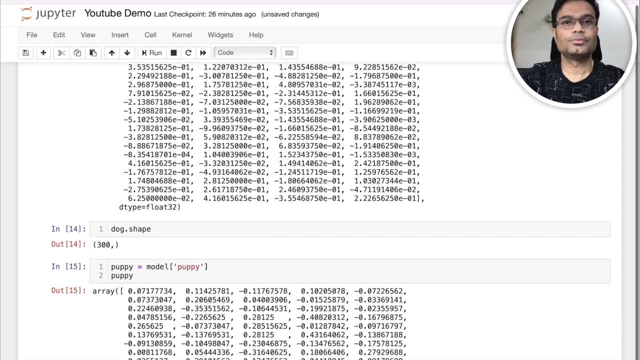 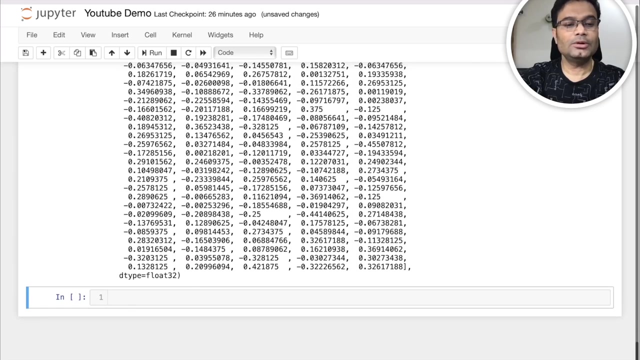 You can see this is almost 300 dimensions. are there, right? The same way we can generate for the puppy also, And then we will see that. what is the cosine similarity for both, right? So when we check our with our data, it was coming 1.1, 0.1.. 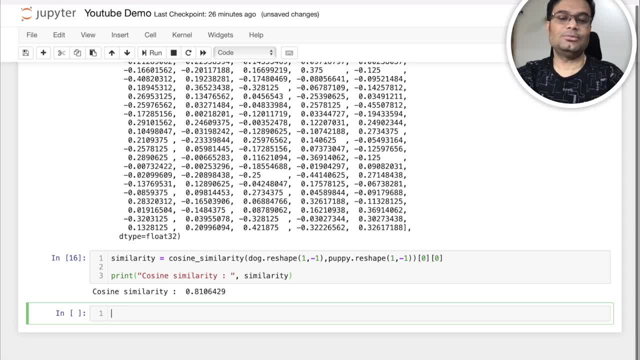 Now, if you see with this shape of this one, you can see 0.8 is coming, because they they preserve many more context information, because they have the predefined user corpus things right. So now we can see the similar kind of things. 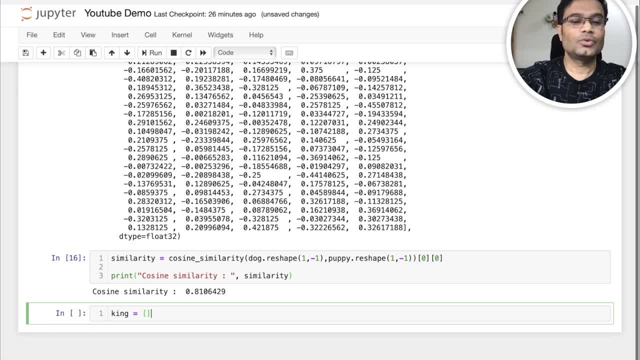 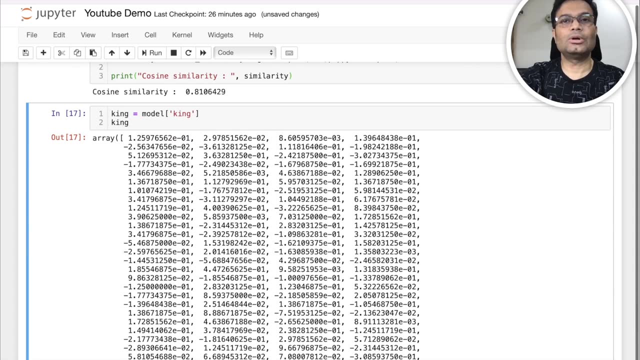 Suppose, if I want to see what is the embedding for the king, right? So go model and put the king: Okay, This is embedding for the king, right. Why I'm doing for the king? because you know we have the one. if you want to know the, 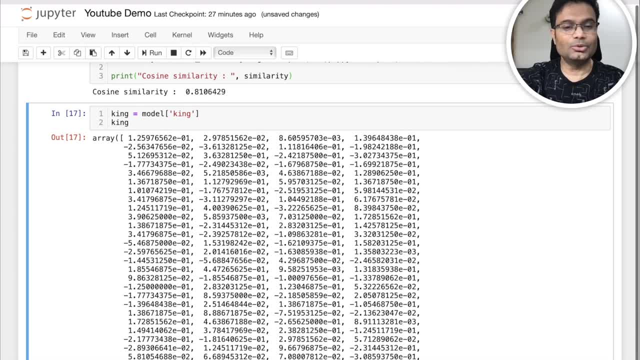 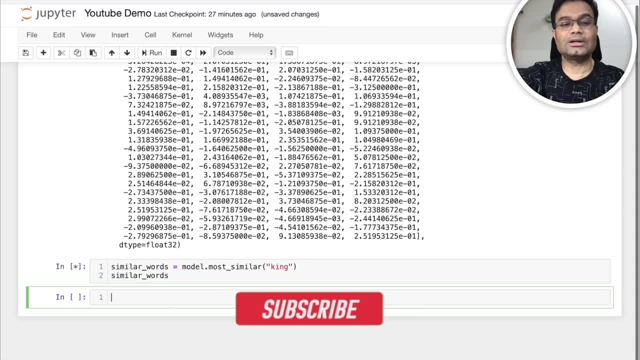 what is the similar data, similar words, as I explained on the whiteboard, If you want to know what are the similar words compared to the king, So you can see that right, So that the similar word for the king, So you can see the kings, queen, monarchs, crowns, queens. 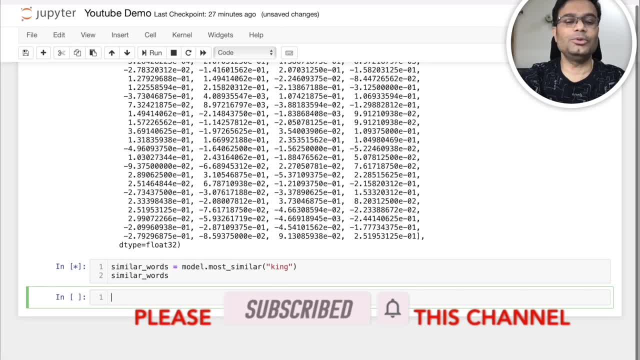 Okay, Okay, The crown princess. these things should be come because these are the similar word for the king. How they able to give the similar word with the help of the word embedding right, So those words also have the similar things, And this will also show you how much similarities are there. 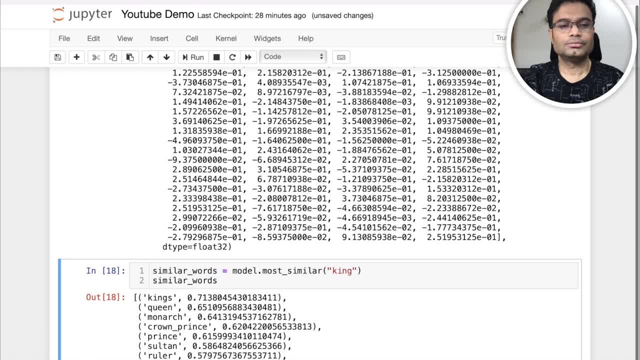 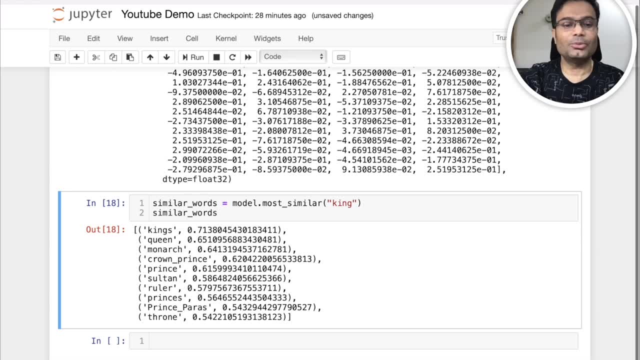 So just to wait for that. so if you can see you generate the similar word for the king and suppose this is the queen, So the similarity is kings. You can see how much symbols are there. This is the way we can take the advantage of the word embedding. 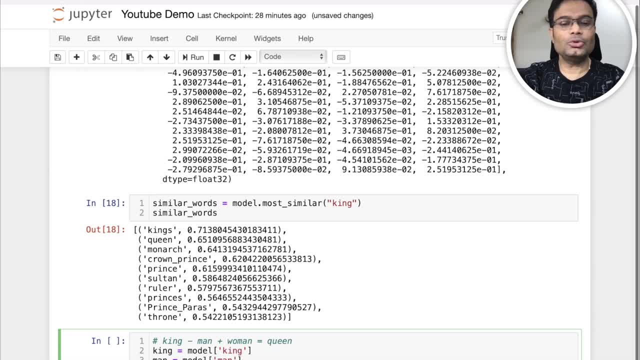 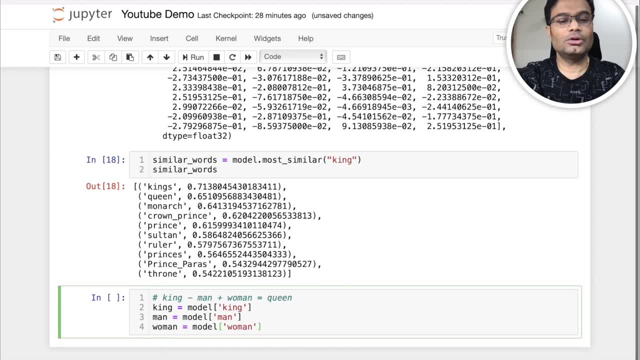 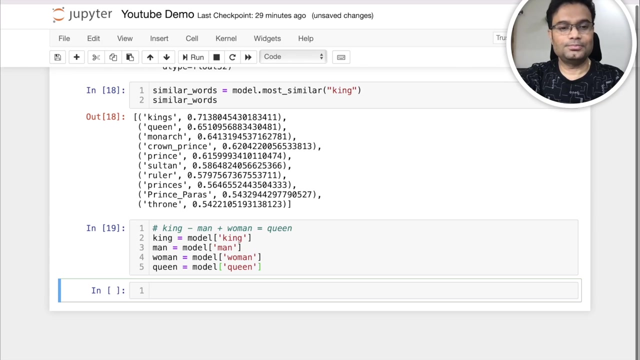 Let me show something very interesting. So I am going to take the word embedding for the king, man, woman, and take also the for queen, And one very famous one example is done. one embedding means if you can do the king minus man plus woman, what should be there? 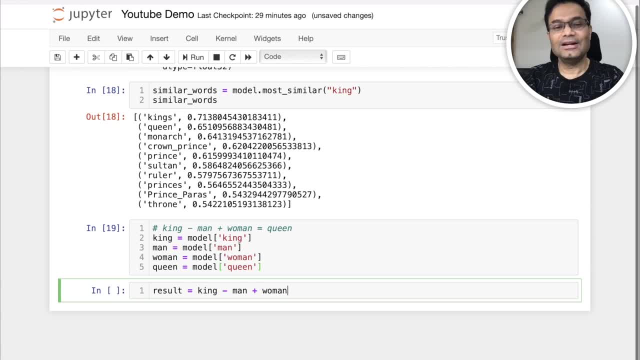 Because if it is a king, right King have the many properties right And if you remove the main properties from the king it become the kingdom kind of things right: The, the, the variety and all those things you can that they preserve. 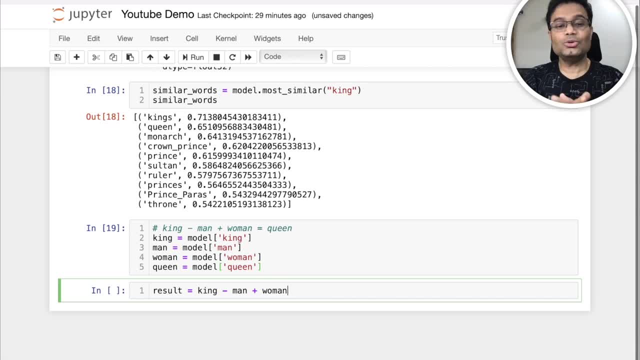 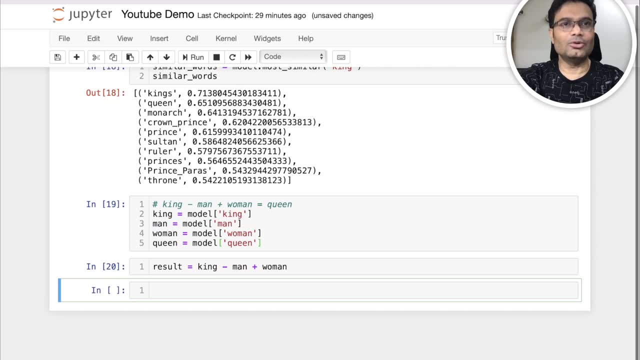 And then on that property, if you add the woman, that should become the queens. So after execute that, let me check that. whether the queen and the king is similar or not means the result and the queen is similar or not. So according to our application, 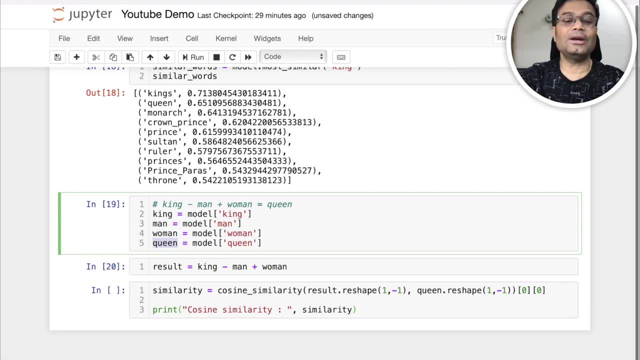 After analysis: the queen- what are the queen? what embedding and this result embedding should be the same. So let me check the result embedding and the queen embedding: how much symbols are there? And if you see it is a 0.73, means it is the symbol right. 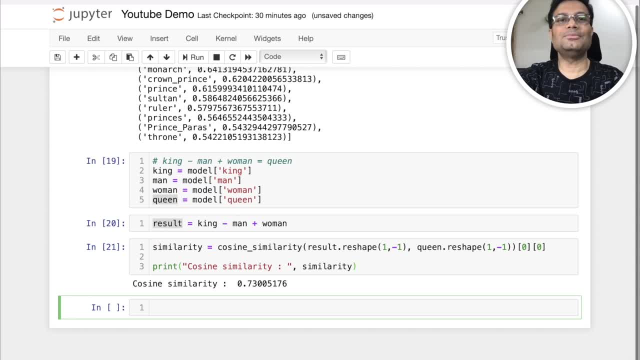 So that's why I can prove that that word embedding preserve the many more things. The same thing, what I will do, the calculations here. you can do the same thing with the different API call. So you can do that model dot: most symbol. 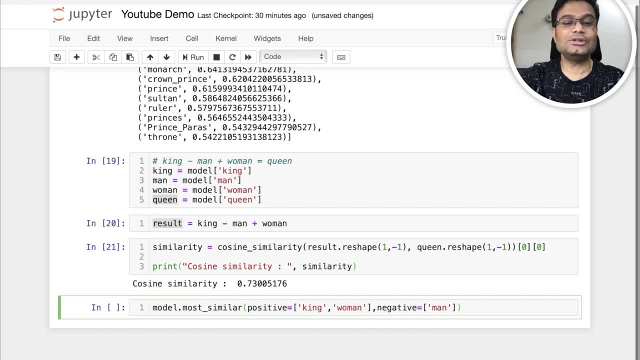 And then you can pass the all. Okay, What are the positive things? Positive means here: king is the first sign, woman is the first sign. So pass the king and woman and what you want to subtract. I want to subtract men. 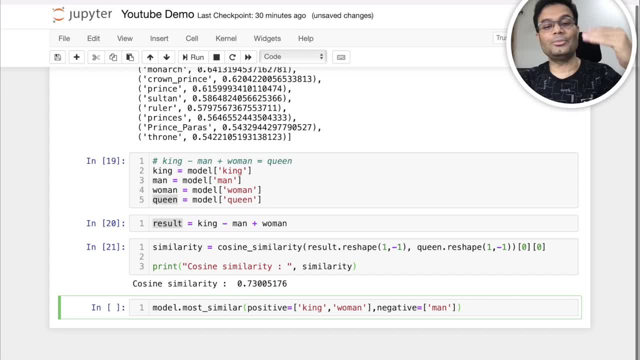 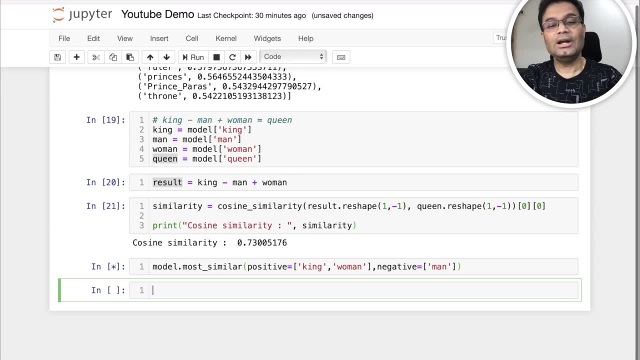 Then tell me, after I add up from king, if I add, subtract the men and add the woman, what are the similarities things should become, Because I know it is a queen and then you can see queen is the one of the result. 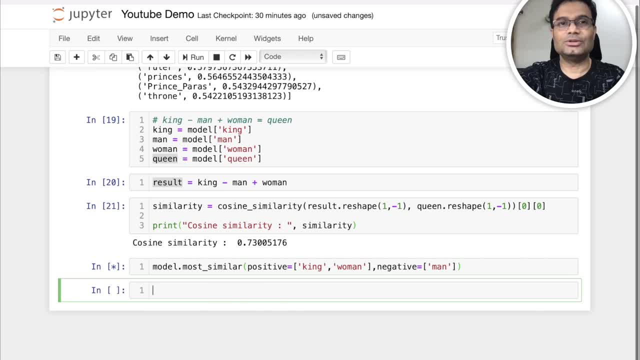 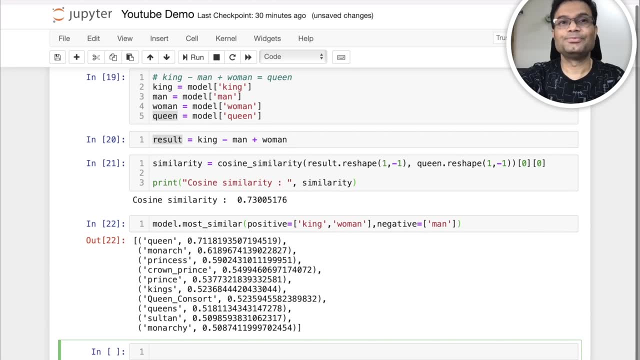 And also with the queen. what are the different results? are there right? So then you can see that here is the queen, princess. Okay, Queen's sultan, monarchy, all those things is coming right. So this is the one thing, and one important thing also I want to show, because this is: